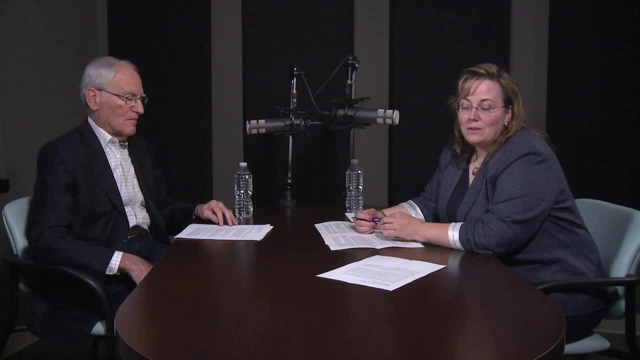 And the creator and longtime leader of Microsoft's secure development lifecycle process. He's also the chair of the US government's Information Security and Privacy Advisory Board. You're a very busy man. Thank you for joining us today, Mr Lippner. 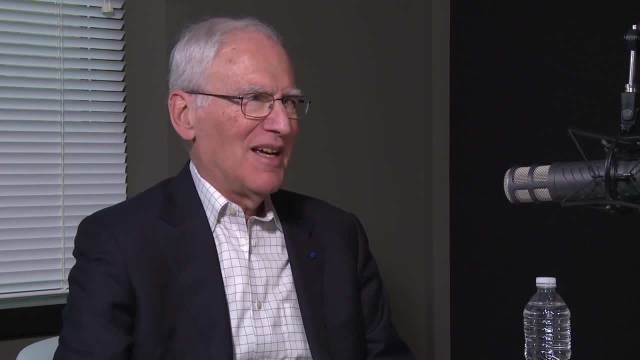 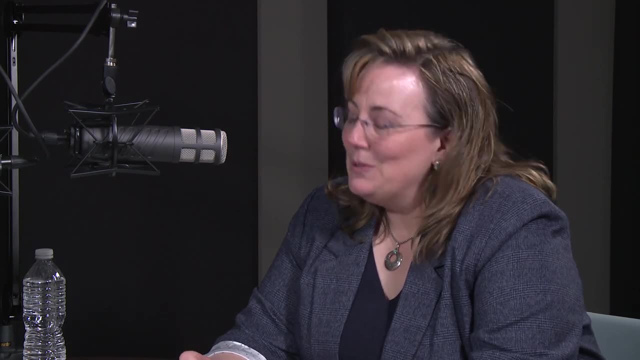 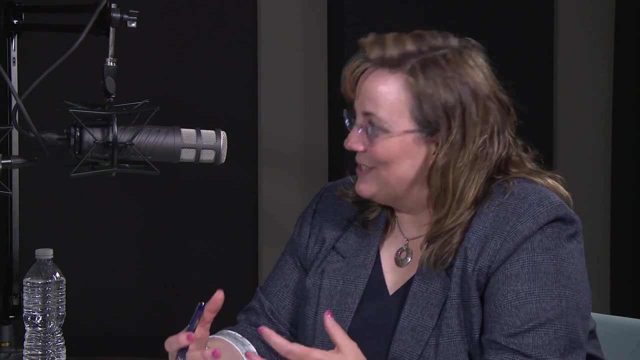 Steve is fine, Bobbi, and thank you for having me. It's a pleasure to be here. It's really great to be reconnected. Yes, indeed, I find the culture of computers and information technology changing so rapidly today, But sometimes we find it difficult to get our grounding, And you've always had your grounding. 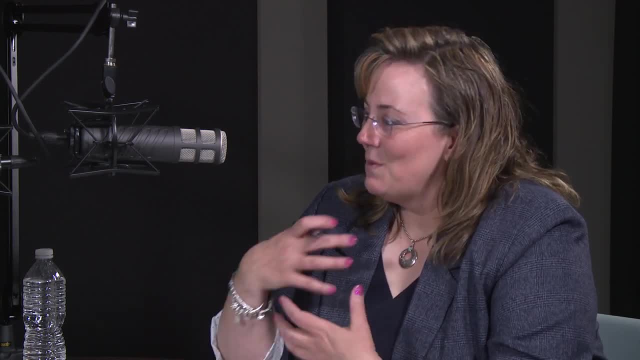 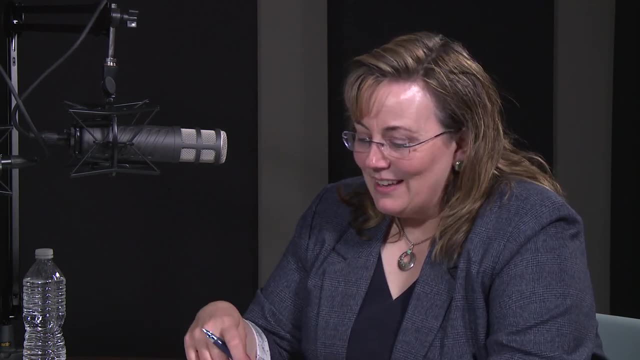 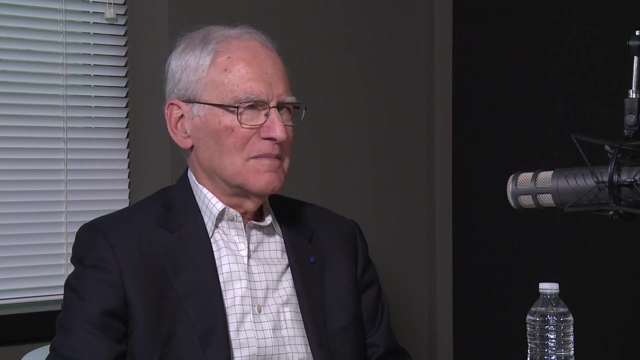 And this podcast is really about exploring the lessons of the past and how we can apply them to the future so that we're not recreating problems, And I think you've got such an important story in this space. You're hyper-focused on software before many others did, And so I really look forward to hearing from you today. 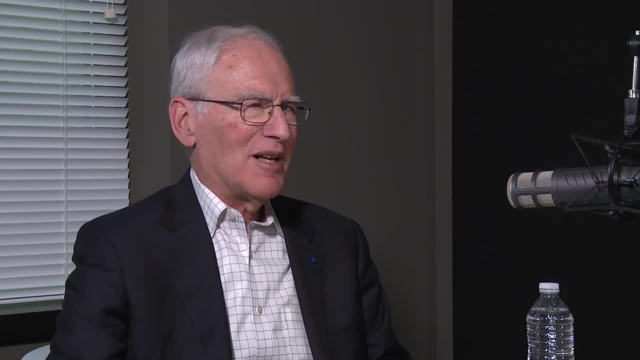 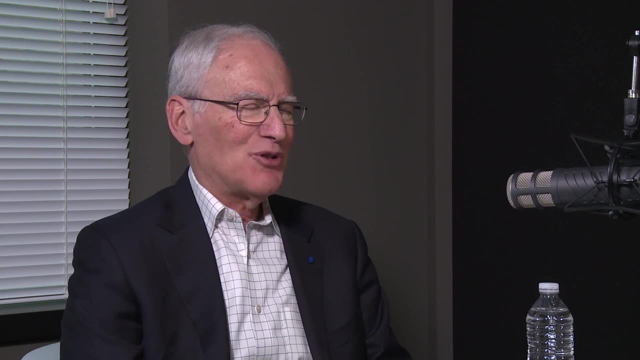 the kinds of issues that you've been working. Thanks very much, Bobbi. It's a pleasure to be here And I, as you say, or as you suggest you know, spent a long time worrying about different instantiations and manifestations of how do you build secure software, finally got into a position and an approach. 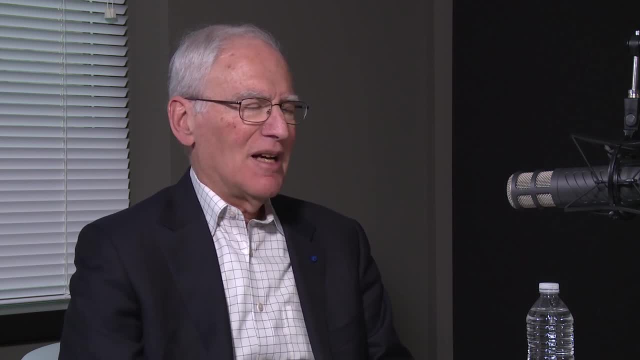 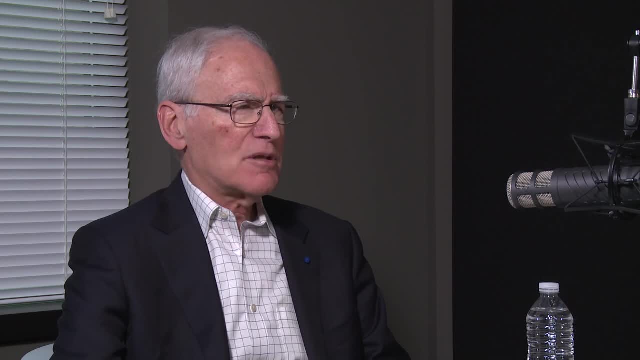 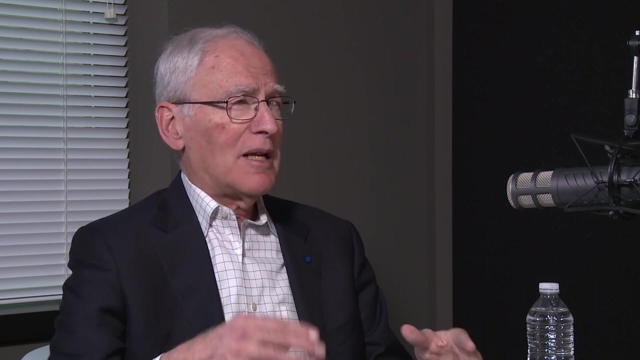 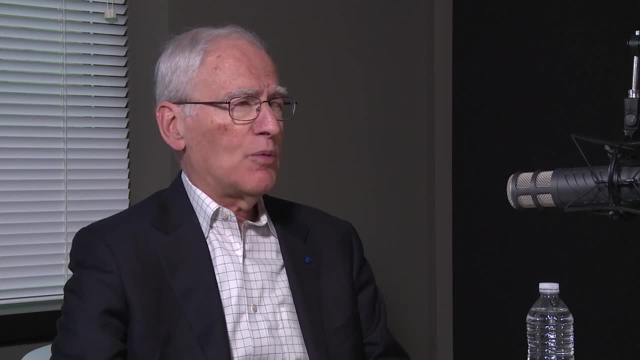 How do we deliver secure software better, How do we get the software we depend on to deliver secure software better And how do we help people be secure so that we're not- we're not- challenged by supplier problems? And how do we? how do we enable the rest of the ecosystem and the industry to understand? 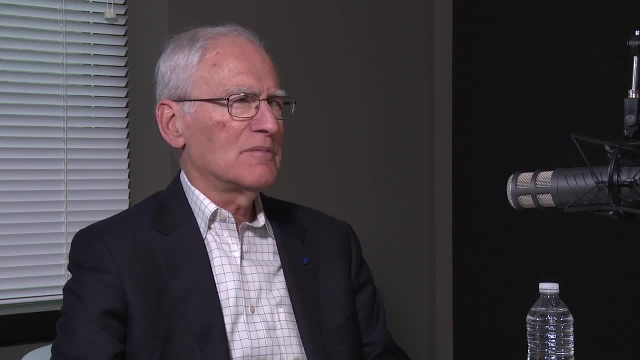 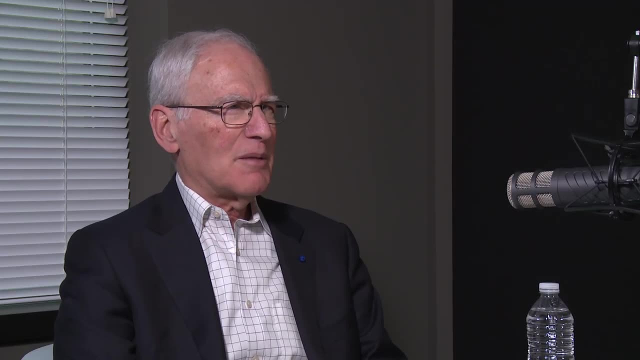 what, what effective and less effective approaches are. So it's a community of the willing to some extent, People who are invested. It's a community of the willing to some extent. I mean, we, we're. we're a small organization. 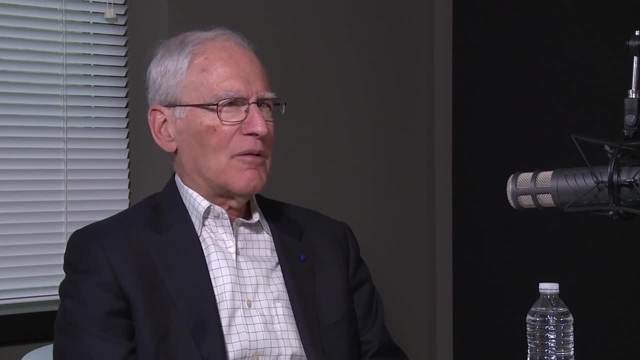 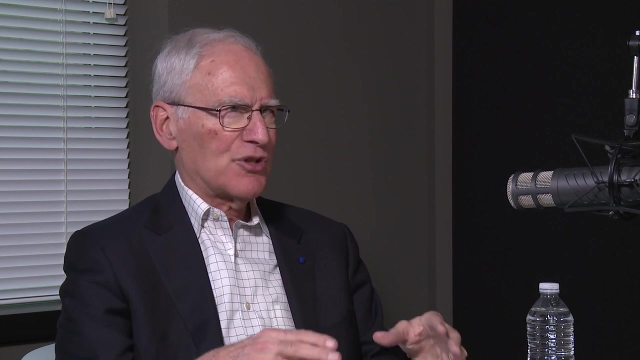 The products and guidance that we produce are are very important. produce are created by the effort of members' employees who band together and work to share their experience and then deliver a common picture of what organizations ought to be thinking about doing as they tackle software security. 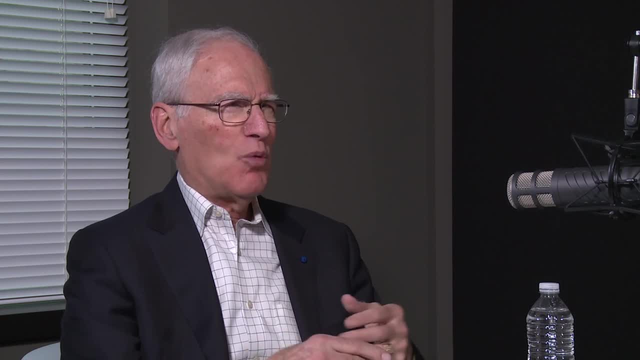 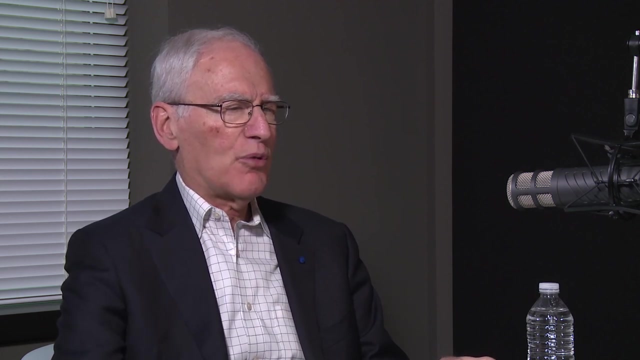 We started out producing sort of heavyweight documents that took a long time to deliver, and there are still some of those very valuable on the website: fundamental practices for secure development, dealing with third party software, how to do threat modeling, or some of the recent ones. 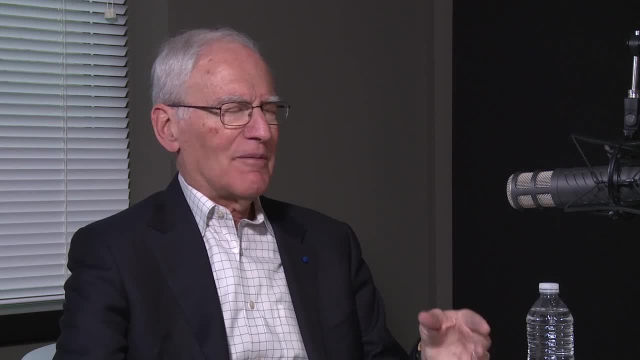 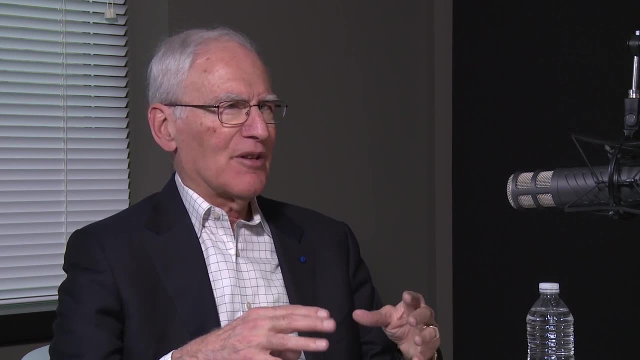 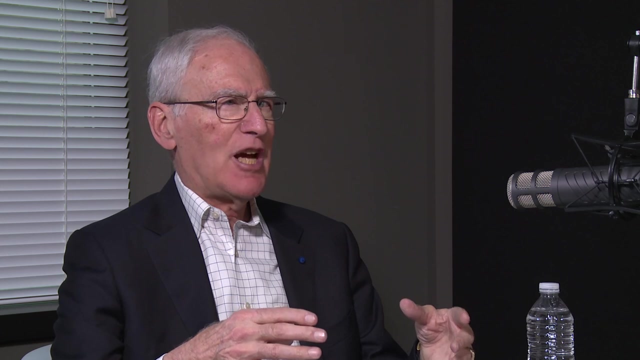 But more recently we've focused on trying to be agile, and so now we're trying to build smaller products that we deliver in the form of blog posts. We did a series of blog posts- One building a security champion program, for example- at the beginning of last year. 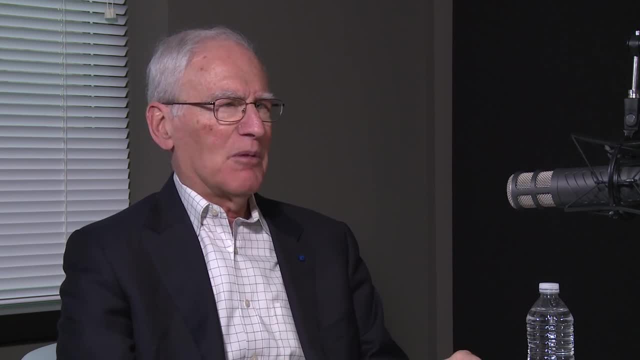 and like half a dozen blog posts over the course of a month to enable anybody who wanted to to say: okay, what is a security champion? why do I want one, and how do I get started rolling that out in my company? So would I be wrong to connect this idea of a security champion to the role you had at 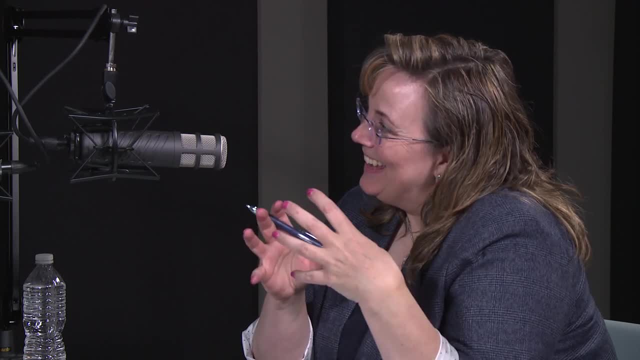 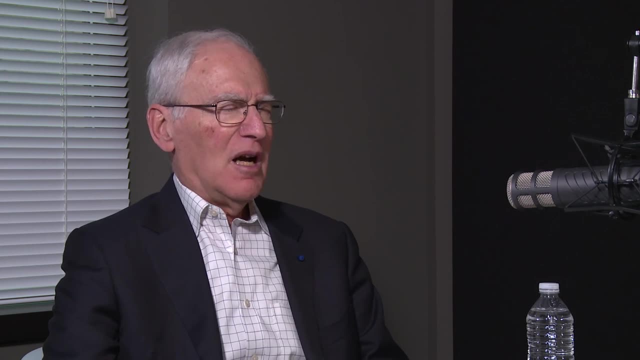 Microsoft in trying to gain advocates to push a secure development lifecycle- You kind of. it's a little different. I was leading what was what we'd call the central security team, the central secure software team. that sort of defined the tools, set the process requirements, manage the training. 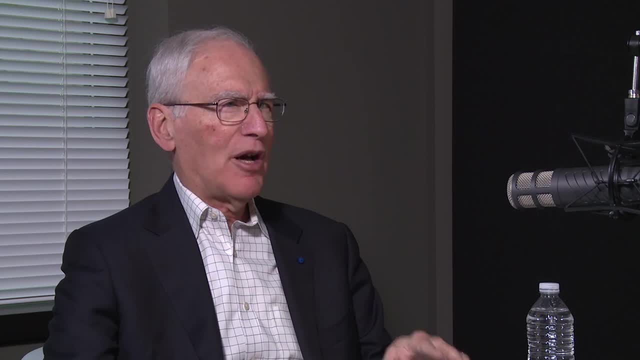 what have you? Security champions are people in a product group who are focused on enabling that product group to deliver secure software. Whatever that product group delivers, whether it's a Windows or a database system or an Adobe reader or what have you- there'll be security champions in the product group engineering. 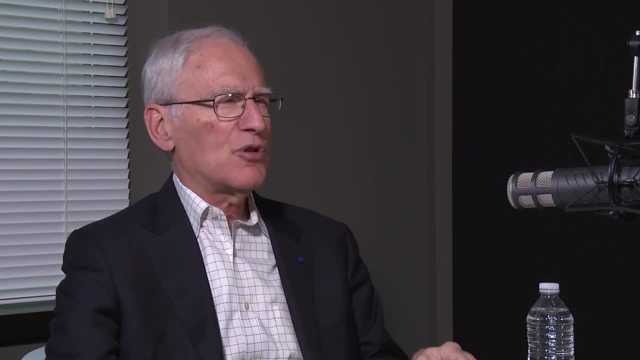 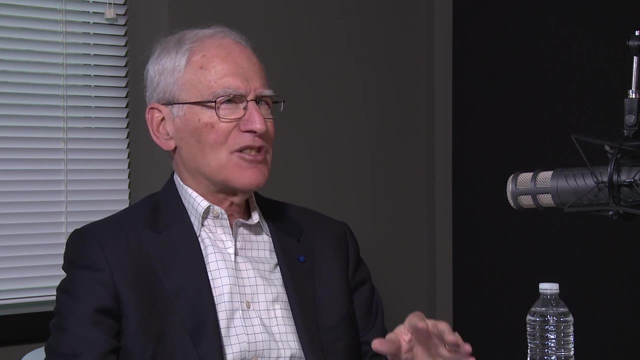 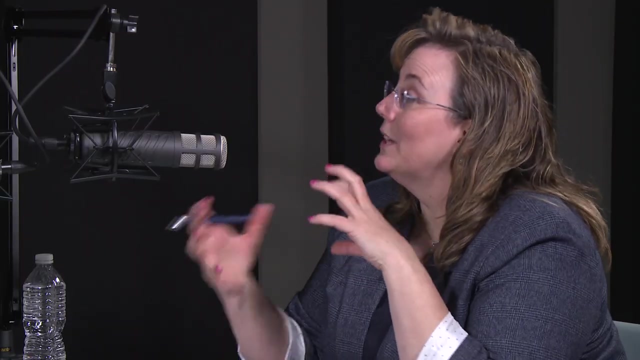 group who are the sort of local go-to experts, local advocates, local interfaces to the broader security program. So that's a very common model in industry and it's worked out very well for a lot of companies. In the Microsoft context. those would be the people you would have worked with in the product. 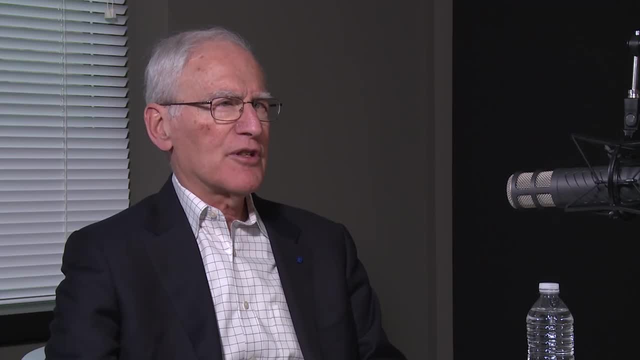 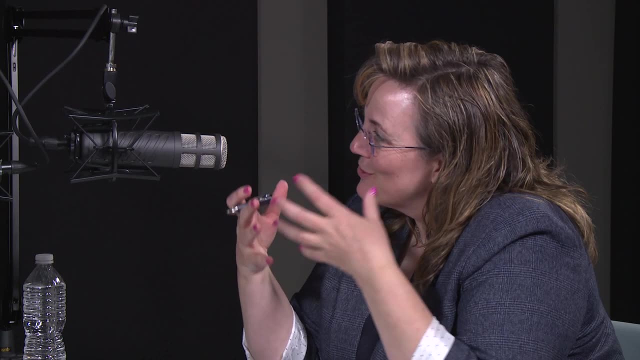 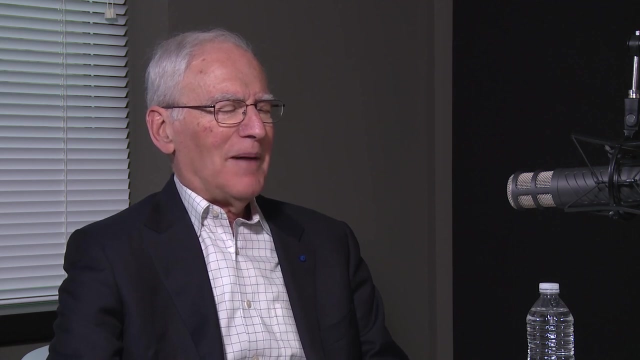 lines that are there In Windows and SQL and Office and so on. So can we talk for just a few minutes about what your catalysts were at Microsoft for trying to step into these security pushes? Well, sure, I mean, back in 2001 particularly, there was just this series of I don't know, I don't. 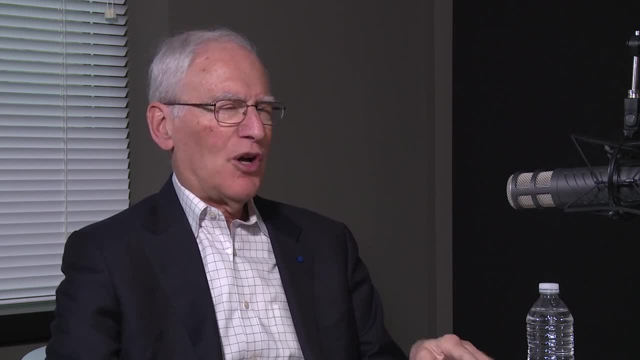 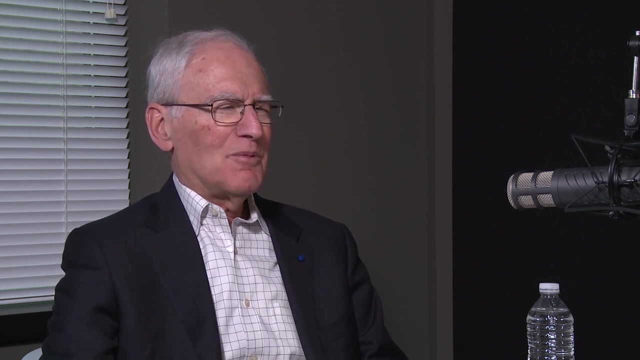 know, security incidents or maybe, if you want to call them security flaming disasters. that's okay too. The code red worm, the NIMDA worm, the UPnP vulnerability in Windows XP, which turned out not to be a big deal, but it got a lot of press. 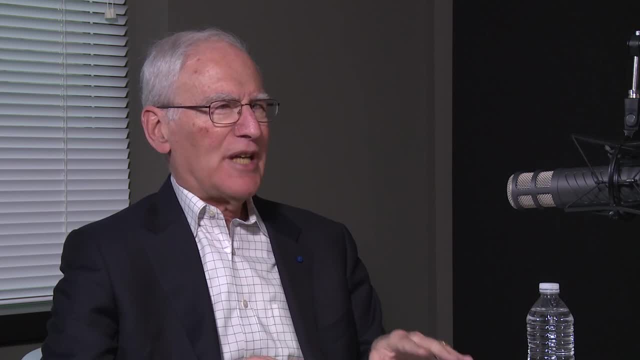 And in parallel with that, customers were yelling at us and yelling at our executives and actually at one point Gartner published an advisory that said: gee, if you're running the Windows web server IIS, you might want to think about changing to another product. 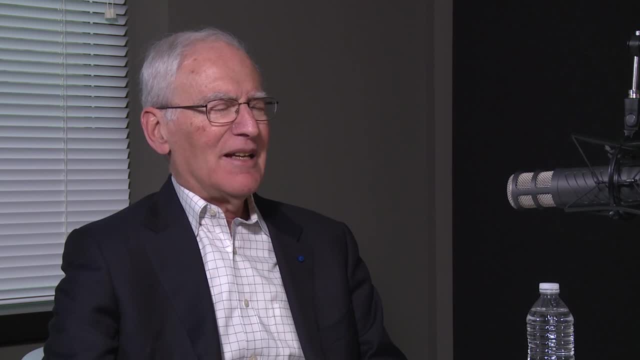 And so that's sort of an attention getter. And internally as well, I mean people at Microsoft took a lot of pride in their work. They wanted to be an industry leader, a technology leader. So all those things came together and really sort of said: you know we're going to do. 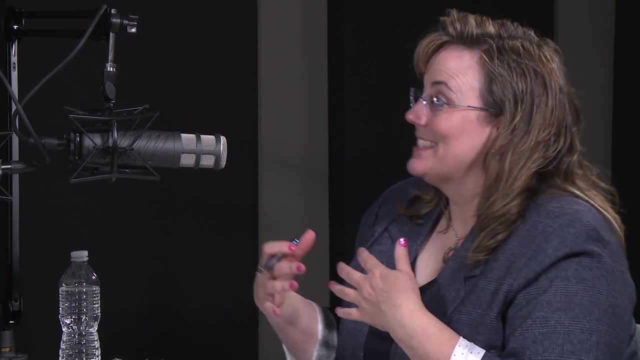 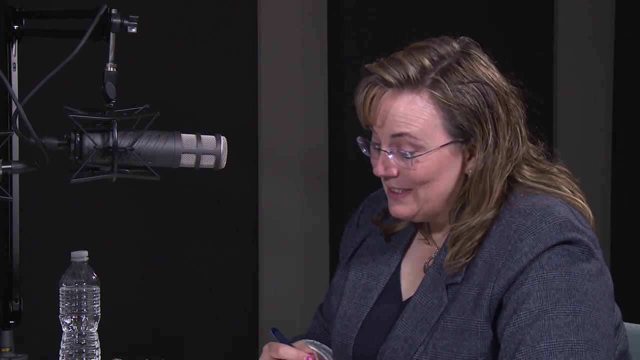 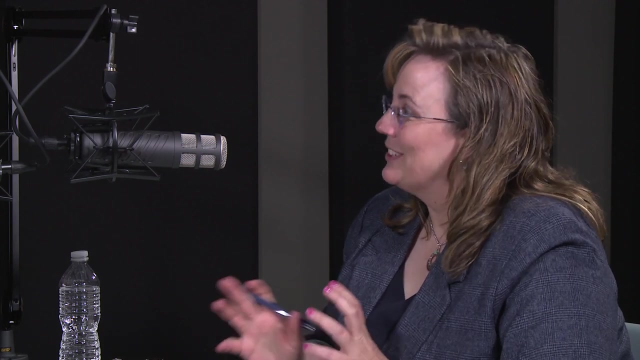 this. We have to do something. Yeah, I was on the operations side of Code Red and NIMDA and others in an ops center responding, So I was certainly personally particularly thrilled with the idea that you were trying to change some of the structure and culture in one of the big products product lines. 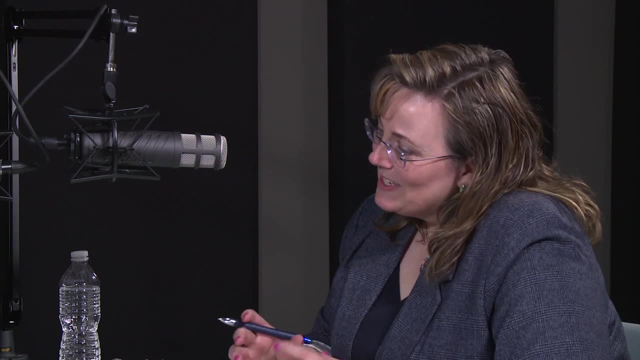 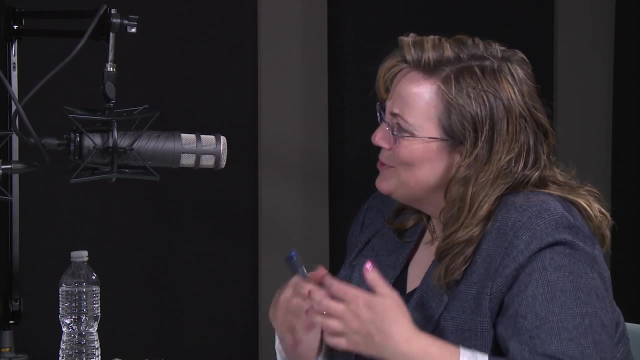 that was out there. So how do you? it strikes me that you've always been an outcome driven person, and I think that's a really important element in this space. right, How did you measure success in Microsoft as you were taking this on, and how do you think? 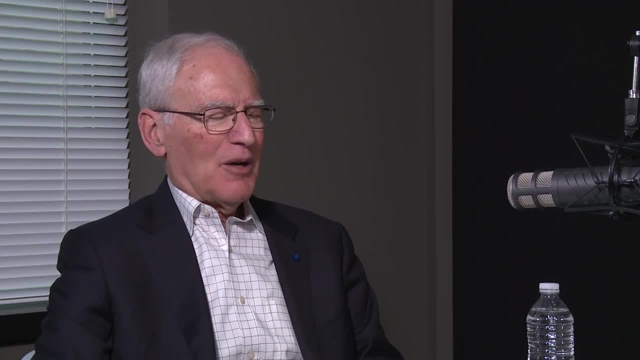 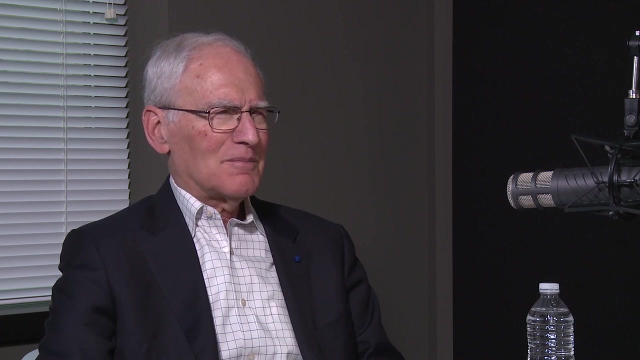 about that today. So there were a couple things. I mean, you know you want the product to be more secure, but we don't know how to measure that directly And in fact I was talking to a professional colleague- pretty well-known vulnerability. 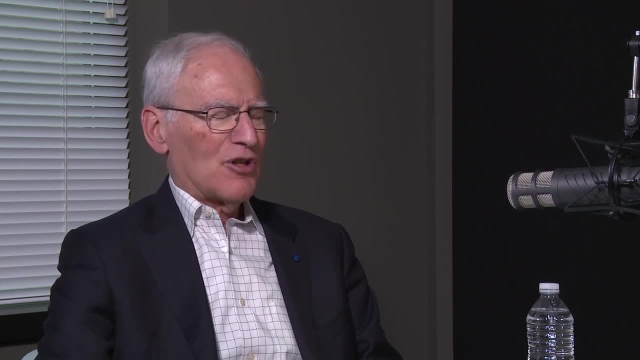 researcher about. you know some of our, You know some of our efforts over the years. this was probably four, five, six years ago And he said: you know you guys have done a good job and I know you've done a good. 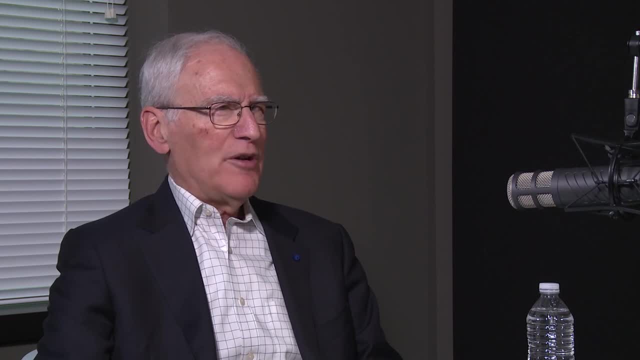 job, because the free market price of a Windows zero-day vulnerability has gone way up from what it was 10 years ago, And so you know that just to me, I mean you're absolutely right and it is a metric, It's an outcome driven. 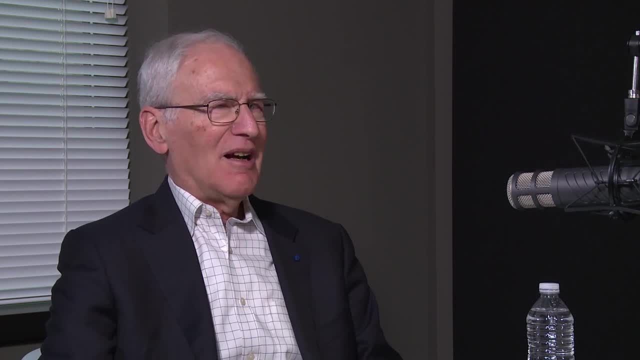 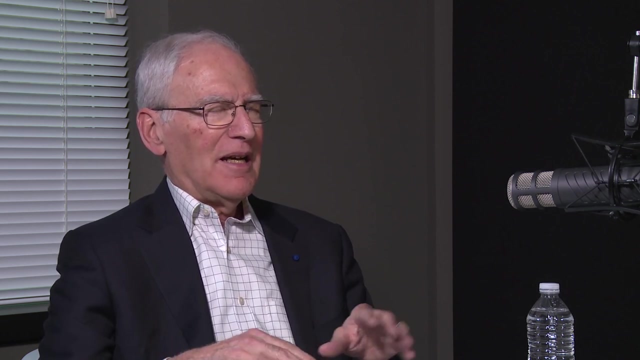 It's an outcome driven metric. It's not one we can cook, could cook and you know, but how do you? you know? short of that, how do you measure? What we did was really two things. Number one: the requirements that we put in our secure development processes were really 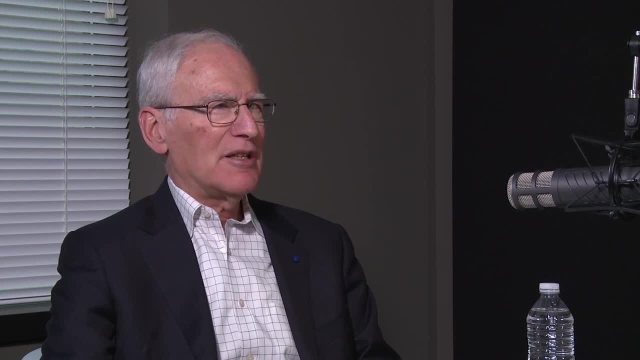 driven by experience of vulnerabilities. So you know how do people attack our systems successfully. And then those requirements are explicit enough so that you can tell very clearly whether the product team has in fact met those requirements. I mean, if you look at the copy of Microsoft SDL version 5.2, that's a free download on 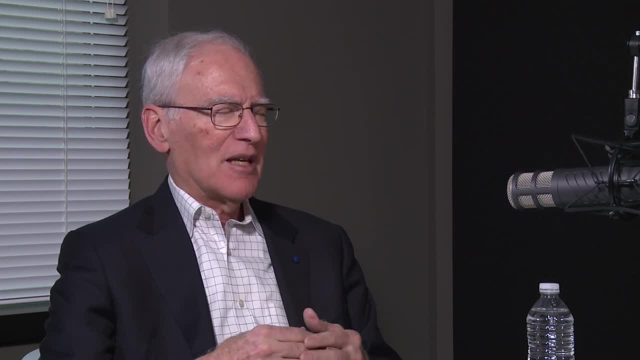 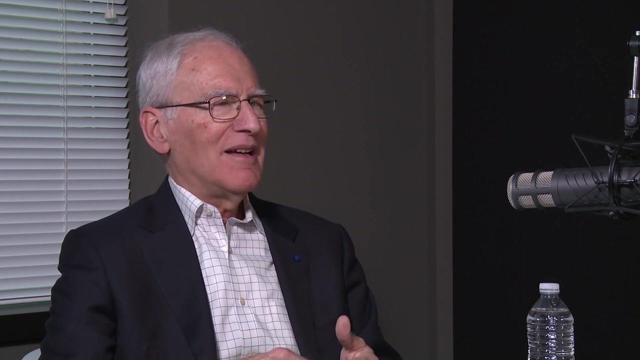 the web and you look somewhere. I think they may be in the appendices. but there are specific static analysis tool bug numbers that are must fix. Okay, And so you know that's measurable, It's cheap to measure. You run the tool and it tells you. 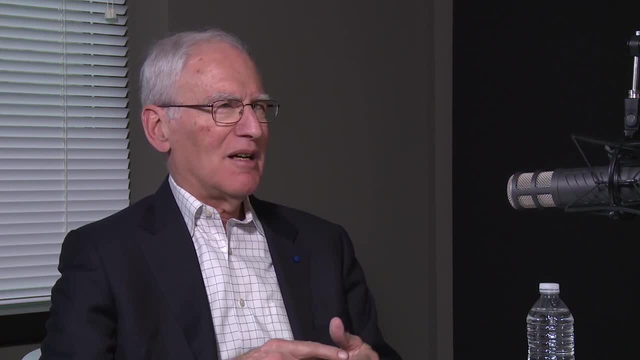 It's cheap to measure whether you've gotten all of them. You just do a query in your bug tracking system and it'll tell you, And so that's meeting the requirements, And then the requirements to actually improving security. that's driven by experience with. 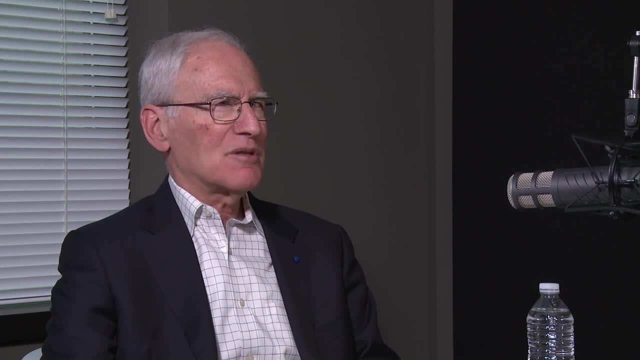 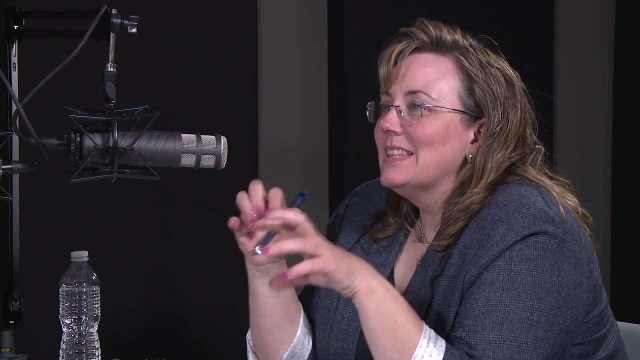 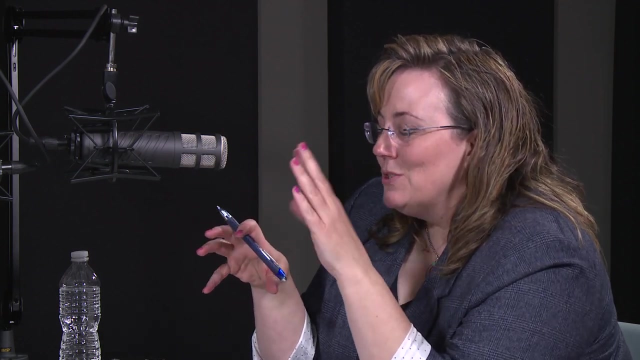 vulnerabilities and experience, Okay, You know, having to fix or not fix vulnerabilities going forward. The interesting thing about those two examples- and I think one of our struggles in measurement- is that on one hand, your requirements, the people doing the measurement have the ability. 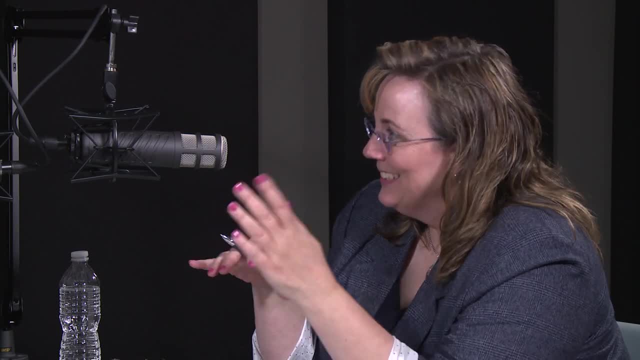 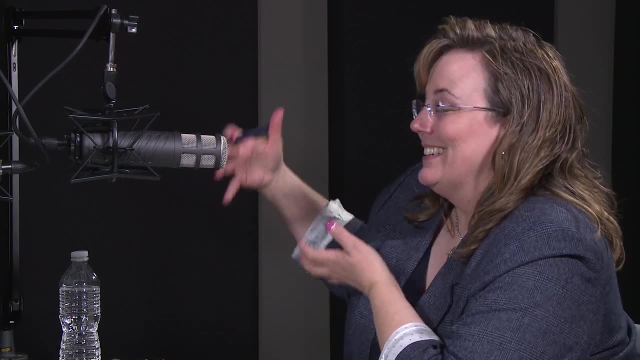 to see the link between their action and their result And that outcome measure. you can't you know that's measured by someone outside of the organization. I think that it's a really useful outcome measure, but bringing it back in and showing 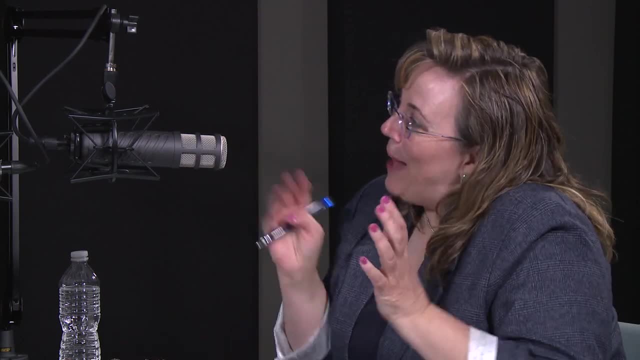 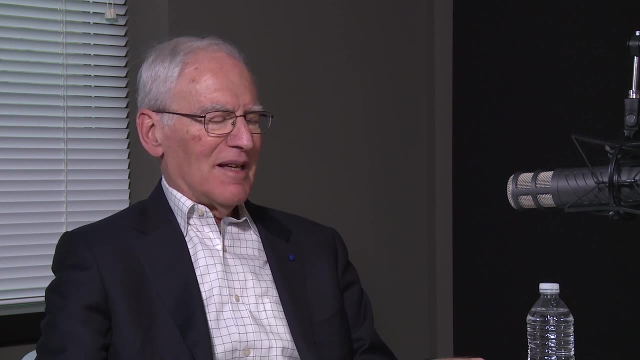 what actions complied. that's sort of the gap today. So you can say: well, you know there's some sort of an integer overflow, that somebody you know attack, you know vulnerability, somebody's going to write an attack and exploit. 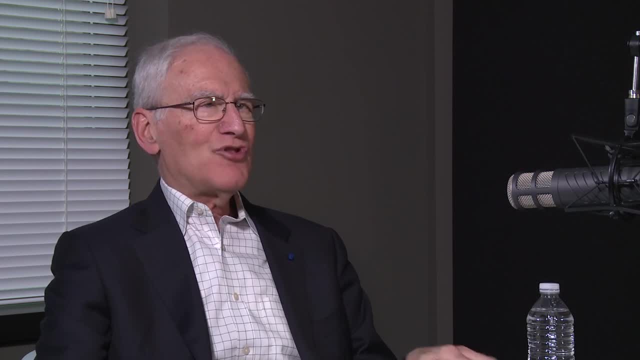 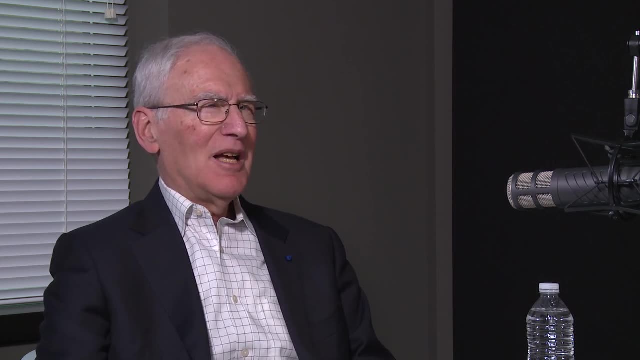 it and some terrible thing's going to happen. So if I had only just fixed that one, you know, then, you know, then things would have come out much better. But you can't. you know, in the security world you just can't attack it that way. 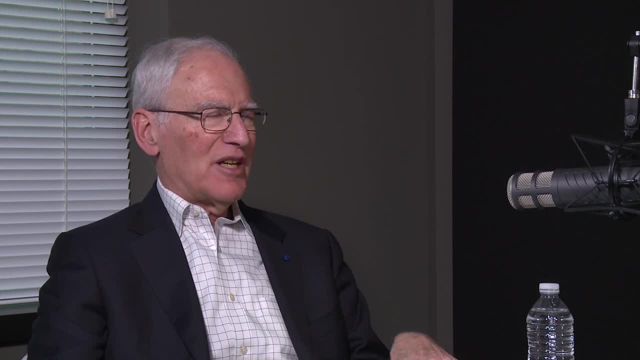 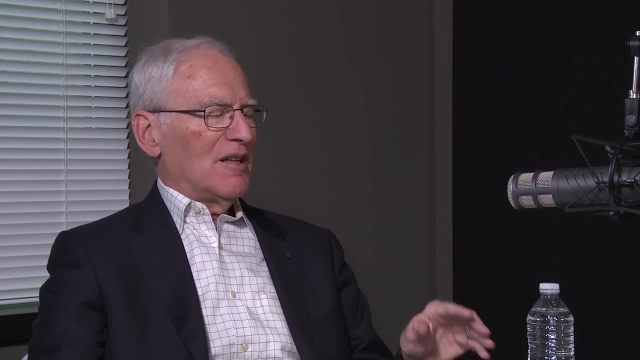 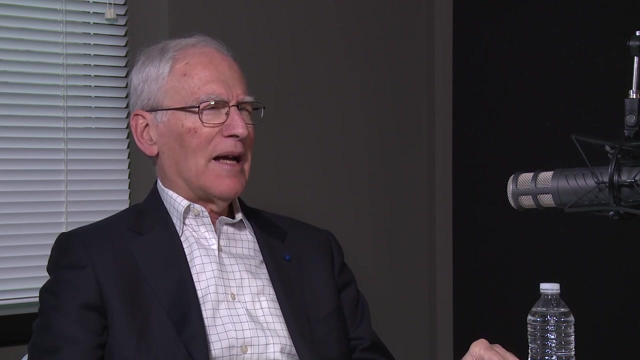 I mean Michael Howard, you know, who co-wrote the SDL book with me, and one of the key developers of the SDL. at the beginning, you know, he used to say: you know, just fix it. I mean, you know, don't not a matter of you know, trying to second guess whether somebody 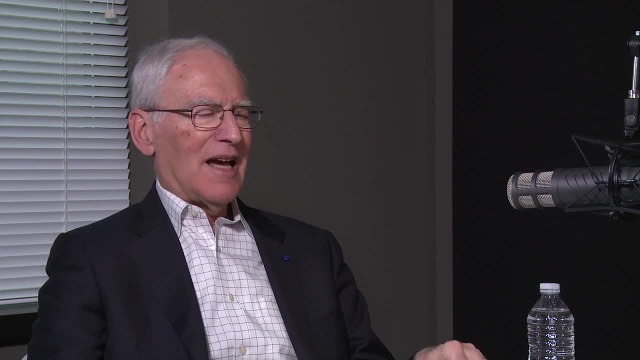 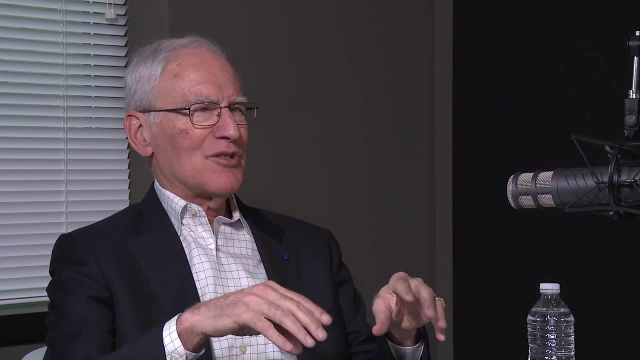 can exploit this, Not a matter of trying to second guess. you know whether we're going to be able to. you know whether it's really a vulnerability or not. you know if it violates the requirements, just fix it and then you won't have to worry because probably if you try to guess whether 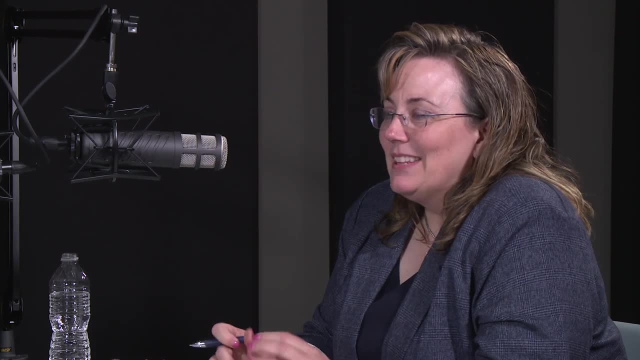 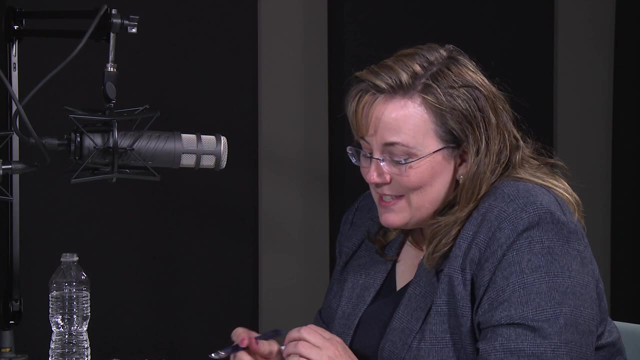 it's exploitable or not. you're going to guess wrong And at some point the energy spent to that could be better applied to just the fixing it in that space. So you've said that security assurance has been the most challenging topic I've had to. 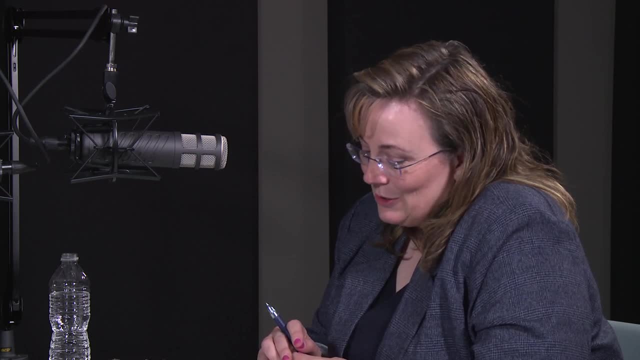 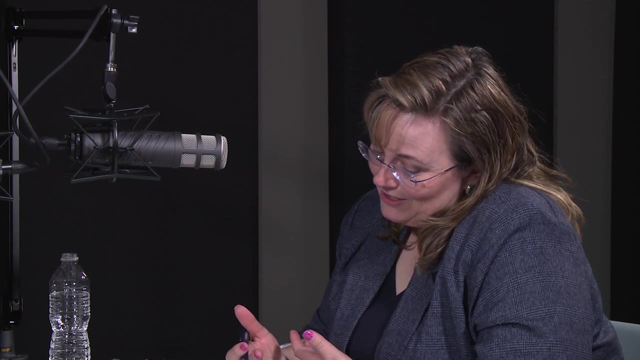 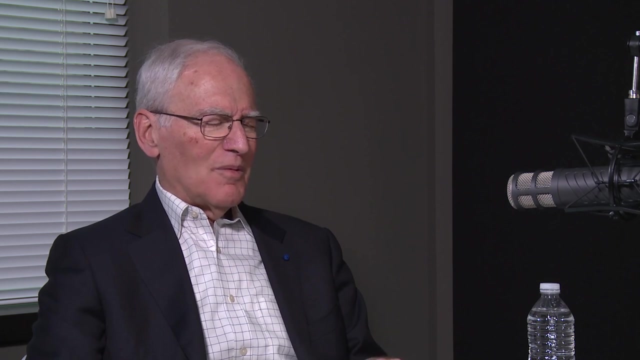 contend with in my 45 years working on computer security? Why And how have you thought about where we are relative to methods and processes and formal validation? Well, so you know why. why is it? why is it challenging? because it's it's really. 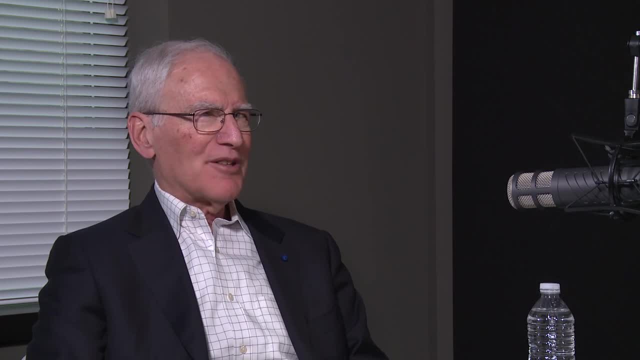 it's really adversarial. I mean it's really an emergent property of systems And so you know, you don't. you don't have a clear, Yeah, Definition of when, a of when a system is secure in general. I mean, we, you know back. 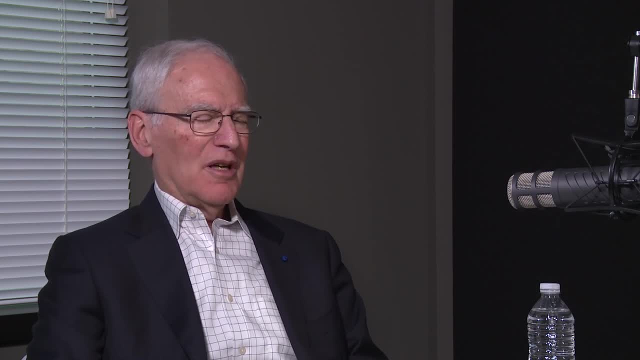 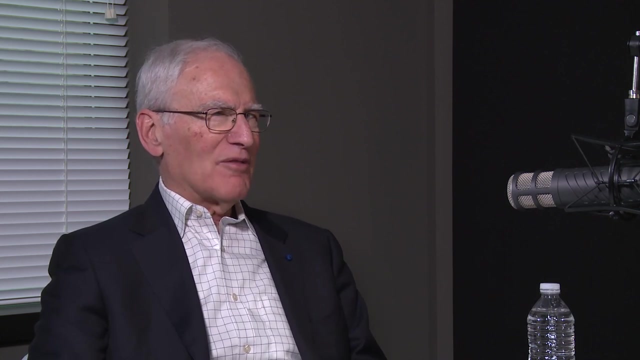 in the in the eighties, a one systems orange book. you know, we we tried doing mathematical models and the- the mathematical models that were tractable- enabled you to build a system that no one usable and nobody wanted to buy, And so that that wasn't very good. 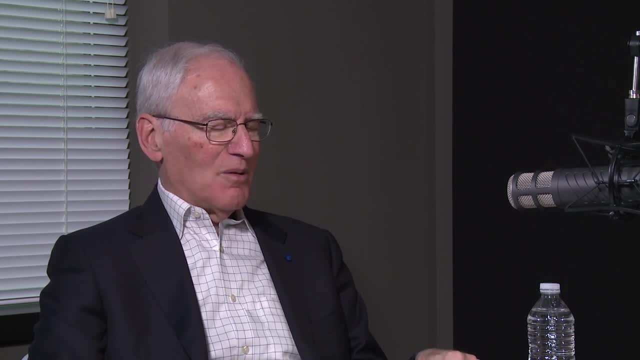 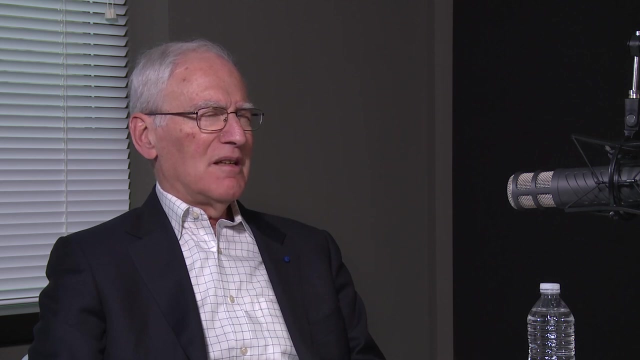 And so you know what? Yeah, So what, what we do, you know. what we do instead is really just to try to say, okay, what you know, be be driven by reality. Um, I mean the Rick Proto, who used to be the, uh, the tech director for information assurance. 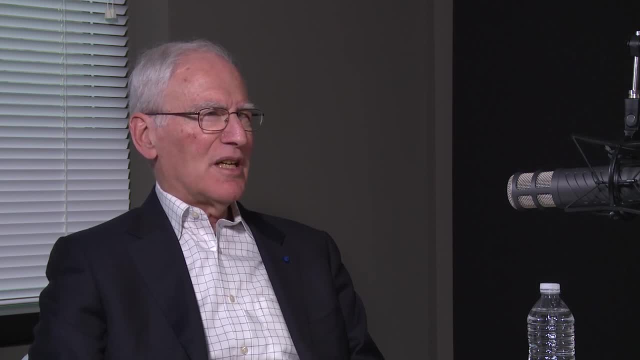 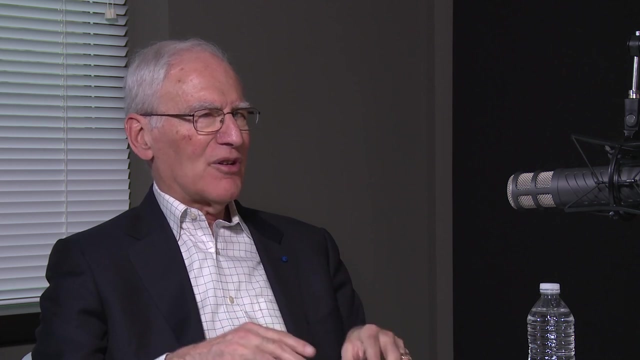 at NSA used to say: you know, theories of security come from theories of insecurity. Start from how people attack systems, And then, Uh Uh, Take that class of attack and frustrated. Take another class of attack and frustrated. Take another class of attack and frustrated. Somebody comes up with a new class of attack. You'd rather they didn't. uh, that's okay, Understand it: Frustrated, Best case. you're good guys, The red team that works for you comes up with a class of attack and you frustrated, and nobody. never knows, it was there. Yeah, They had one fun case, 2005, six um, where some of our really brilliant security researchers internal to Microsoft came up with a class of attack that was really pretty bad. uh, pretty pervasive. 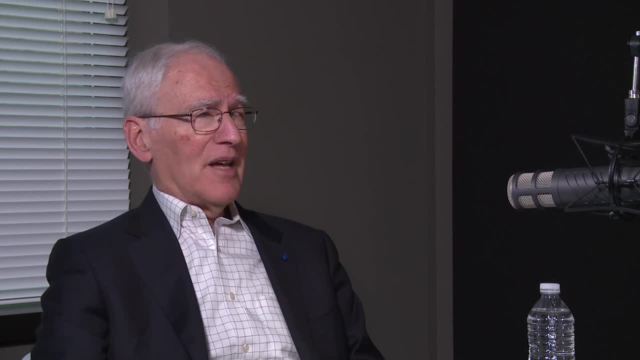 Uh, and then they, they built a tool that that enabled us to find uh violations of of you know Uh- I'm a scrolling nada by instances of that vulnerability and we made that tool mandatory under the SDL and starting with Windows Vista. we just wiped out all cases of it and nobody. 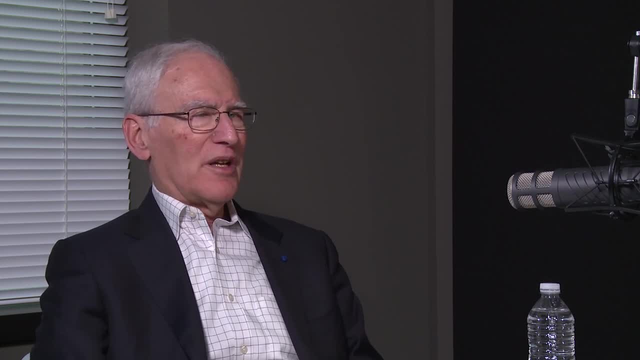 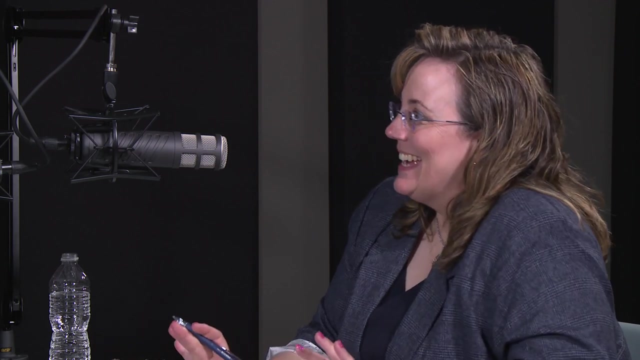 ever knew, if somebody said: you know, maybe for its 20th anniversary I'll get them to publish a paper, but it doesn't matter, because there's no, no system and support where that vulnerability still lives. So that's a beautiful, perfect case, isn't it? 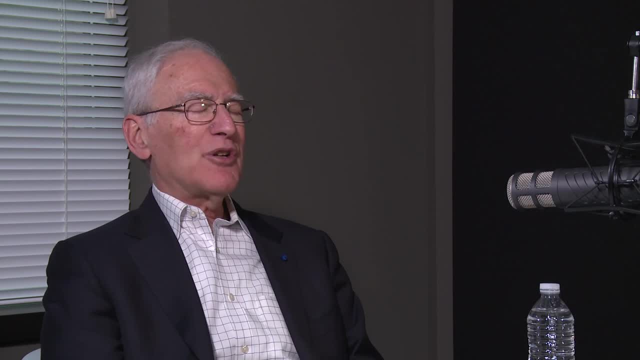 Right, Right. It is a beautiful, perfect case. Everything That's what you're trying. you know that's what you'd like, but you know that case has happened occasionally. Now you know how do you replicate it. 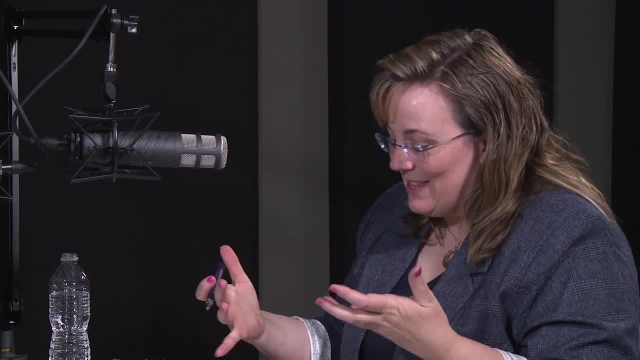 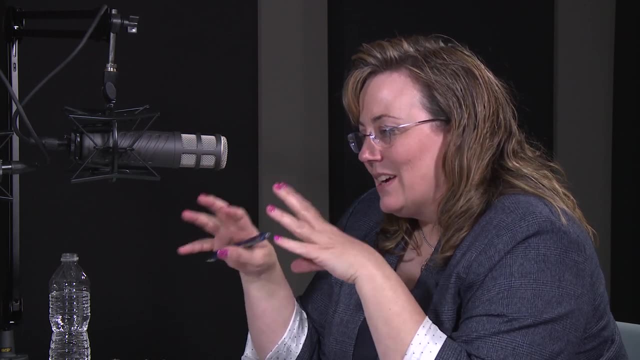 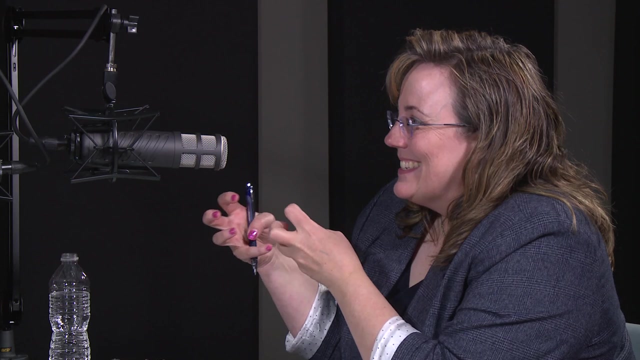 What are the circumstances that enabled that to happen and how do you create those? So, the interesting thing, I'm struck by your language. right, Find a category of attack and frustrate it, compared to this idea of formalism. right, Frustrating is not as precise, you know, perhaps it's just you've made it. 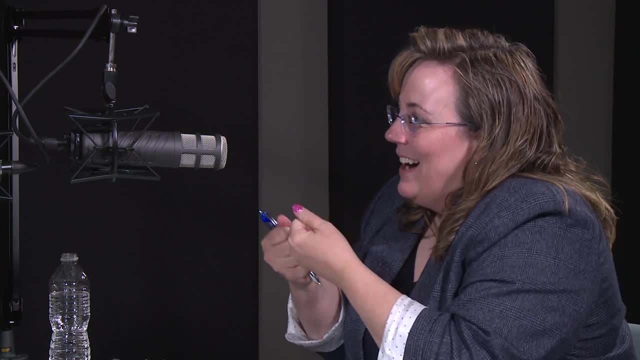 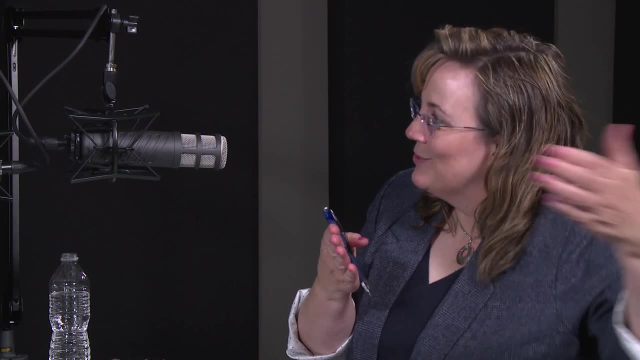 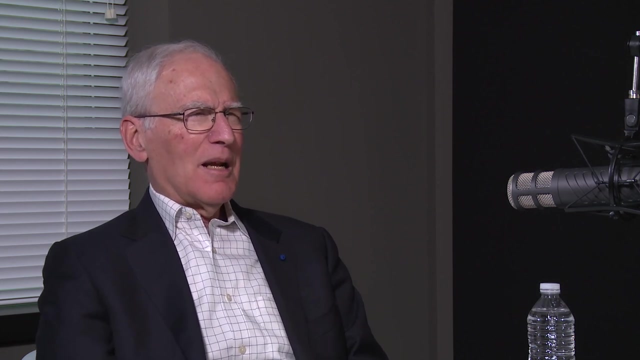 You put so much sand in the gears that you've moved beyond the adversarial move beyond compared to what's the level of formalism that verifies that you're not going to have something. Was that intentional? Not that intentional, but it's probably not a bad model. 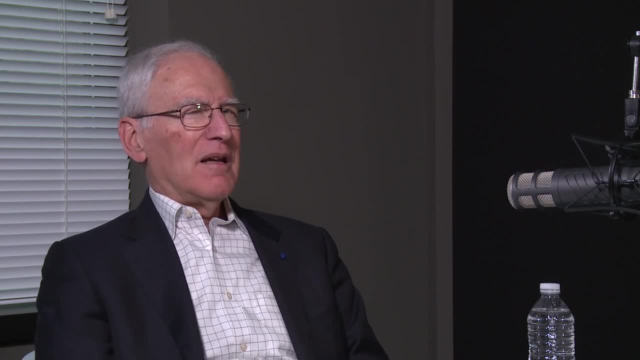 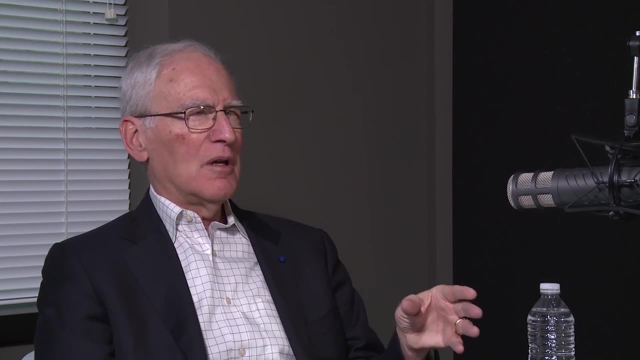 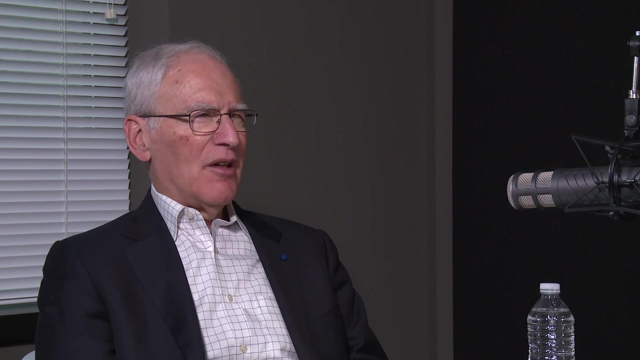 I mean, one of the things we do is to try to So remove, you know, instance vulnerabilities, instances of vulnerable code, when we find them. We we know we're not going to do a perfect job of that, So some of the other things that that we've focused on are what we call mitigations. 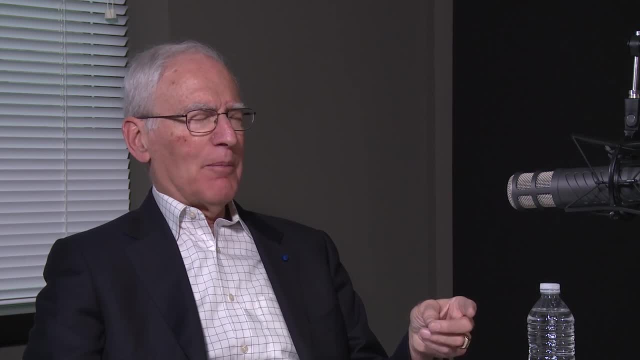 Basically, you know, sort of an old, old example is, you know, 15 years old now, I guess, the non-executable stack and heap memory, Right, OK, I very much remember this. The overruns, the errors are still there, but you can't, you can't, you can't exploit them, or at least you can't exploit them as easily. 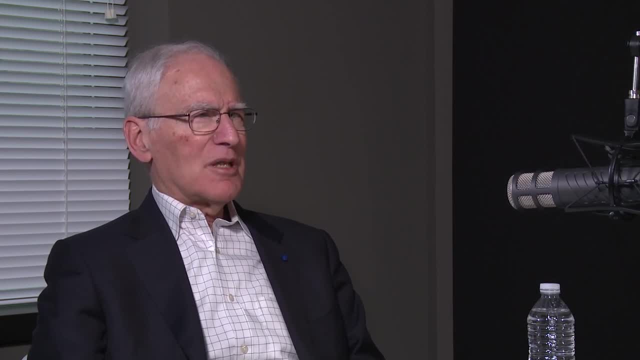 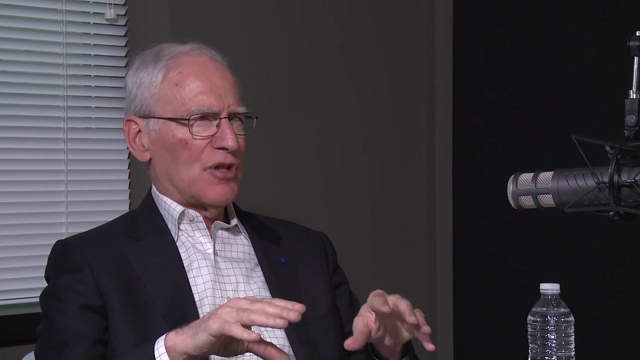 And you know some of you know some of some of the Microsoft, some of the safe code members have done a lot over the years with trying to follow that philosophy, You know, not not as an alternative to writing security Or software, but as a complement to writing secure software. 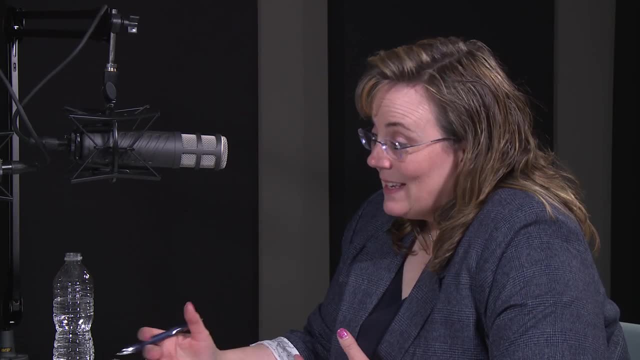 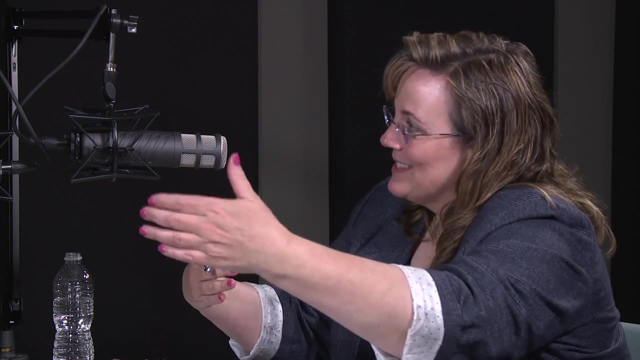 Right. Yeah, it's the interesting thing to me about that example and the idea of a compliment to secure software is the software gets you so far And then at some point the platform has to pick up and that you know how you mitigate the gaps that are caused in that, in that transition. 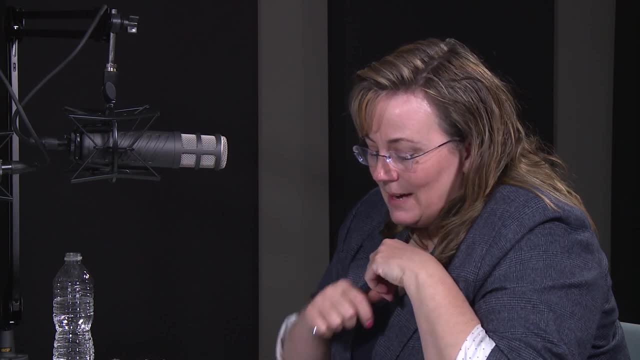 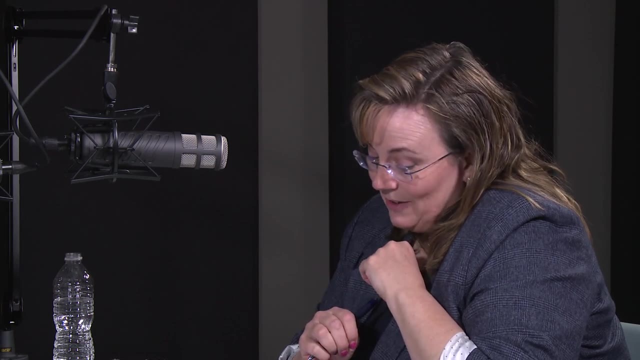 I think that that example is a good one. A good one there Last year it used next 2019.. You said that a big lesson you learned from the role Out of the SDL is that secure software depends on. I'm going to get this right. 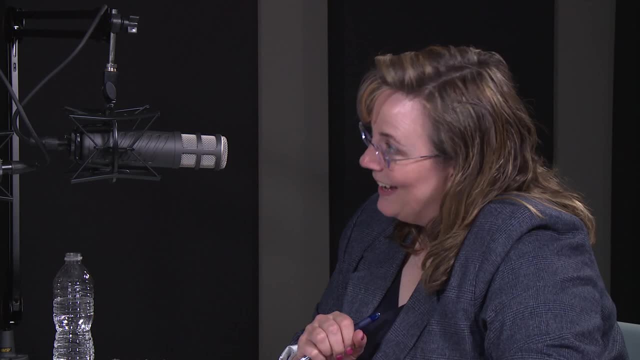 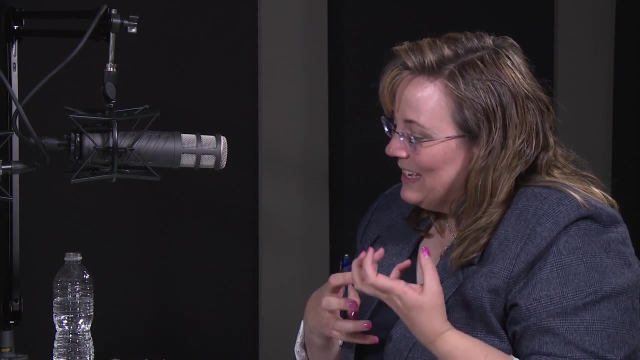 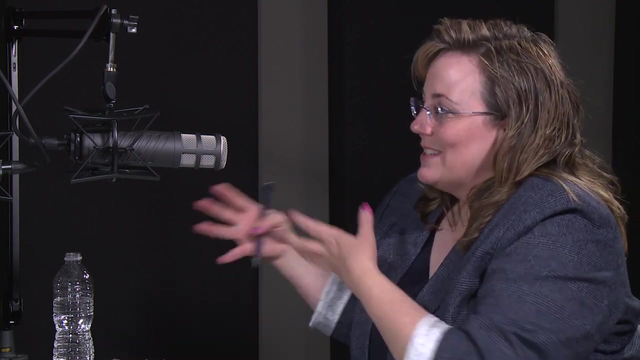 Enabling secure development. rather than measuring security compliance, We keep trying to compliance in security. How do we think about, how does your experience help us think about, not taking that tact in the future? Is there some lesson from that that we should? I think? I think there very much is. 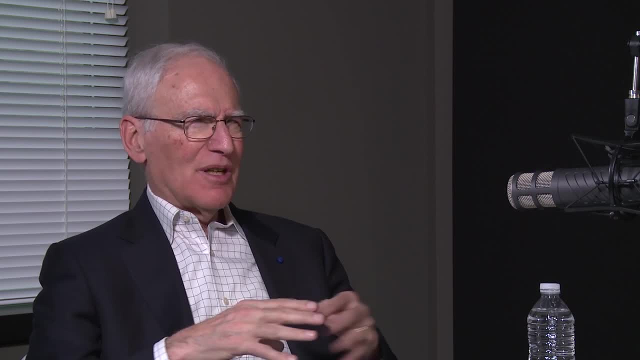 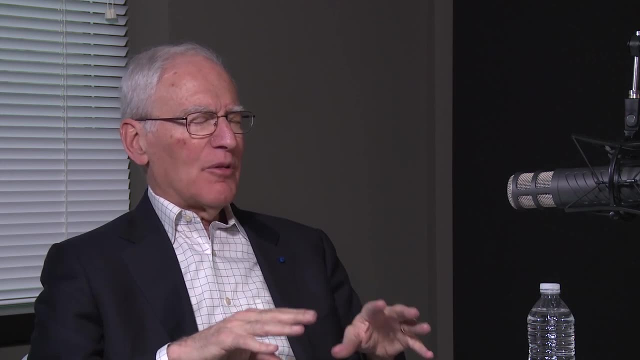 And that really sort of goes back to the history, History of the, the, the Windows security push. OK, we, you know, at the time of the Windows security push, my team, you know, that was sort of driving the security push, was was like four or five people. OK, eighty five hundred Windows developers- OK, the numbers didn't write. We're not going to review all the code and find all the security bugs, although I think that was a model at some point before I joined joined that team. But you know what? what you can do and what you have to do is to motivate the developers to write secure software, train them on what that means and then set them loose to doing it and provide tools, training. 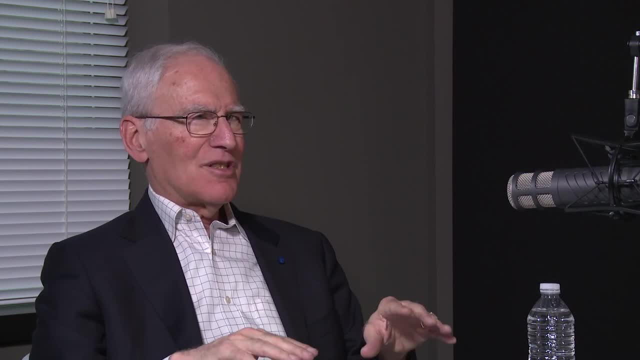 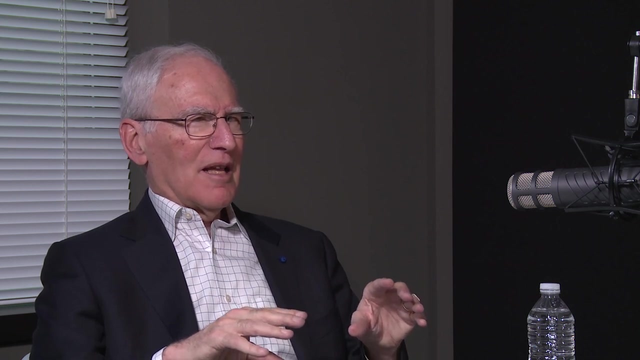 Process best practice. This is an advice when they need it and that's a, that's a scalable approach. if you, if you say I mean I've literally seen companies- and I think all, I think all our safe code members are past this- literally seeing companies, you know where they have a security team, that they have. they say they have a secure development process. They have a security team that comes in after the software is done And then they and then they code review it or they run their tools or they penetration test it, and then they find bugs and then they pass them back to the developers after the developers thought they were done. OK, and so you know, the developers hate that because they thought they were done. Managers hate that because they thought they were ready to ship. You wind up making quote risk management decisions, which too often means I mean, you know, while I can't afford to fix this, I'm going to, I'm going to ship with it. 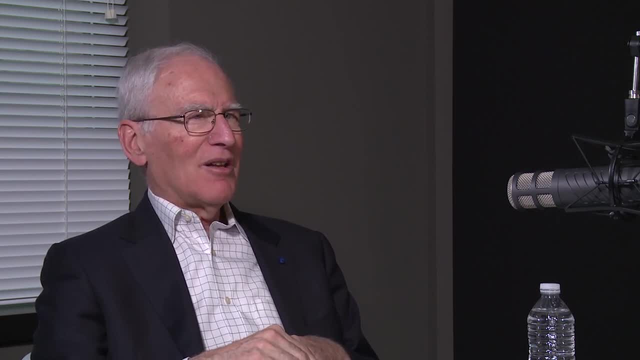 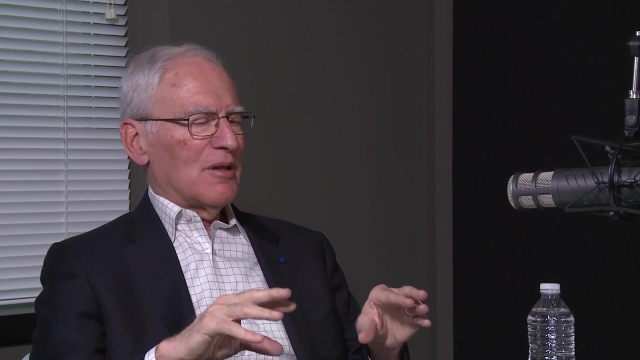 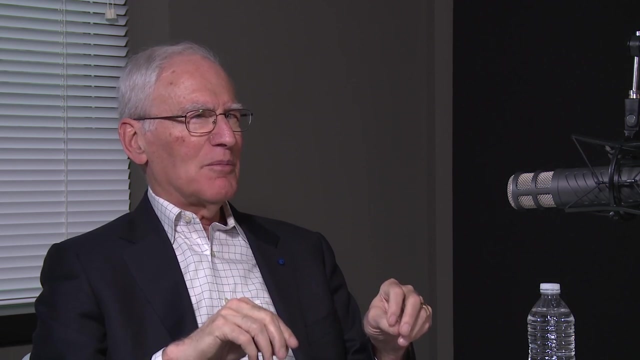 And so you know that that's my model of of what a compliance driven software security program looks like. And you know, and it it it not so good? You know, I mean in comparison, you know, I mean even even the Windows security push. we, we trained people. you know, we gave them tool outputs as they were doing development. And so they, and they knew what code, what bad code, looked like, They knew how to replace it with good code. They came up with an edge case, They, they had somebody knowledgeable like a Michael Howard to turn to, And and at the end we didn't have a perfect product, but we were close enough so that we could ship something that was a lot better than than what we started with or what the prior versions were. 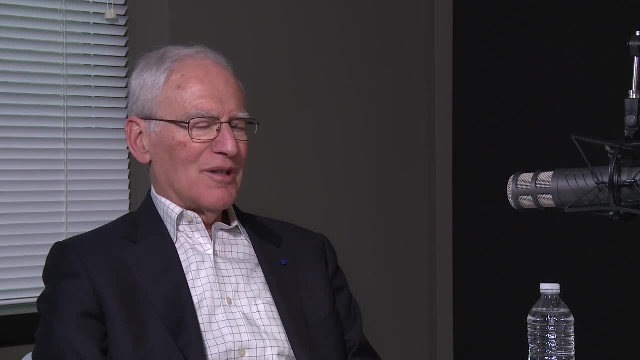 And so that's you know. that's really My view on on on compliance. I mean, you still, you still can measure, but but you know, but the measurement ought to be pretty easy because the requirements are pretty explicit And the tools tell you, and the you know, and the the tools and testing tell you, you know very precisely, you know what you shouldn't have done. 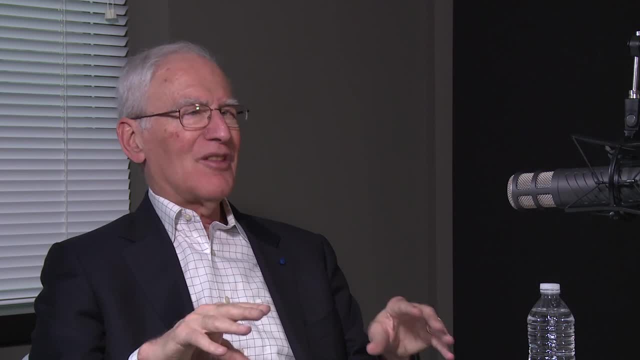 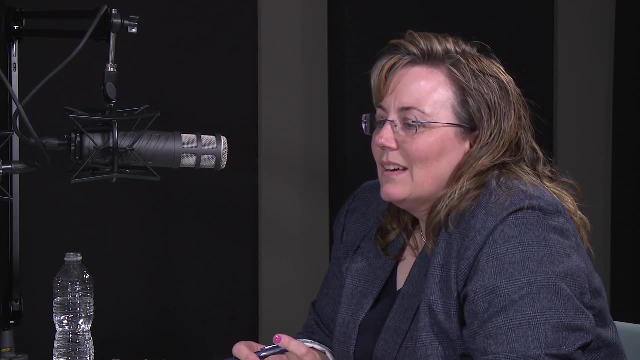 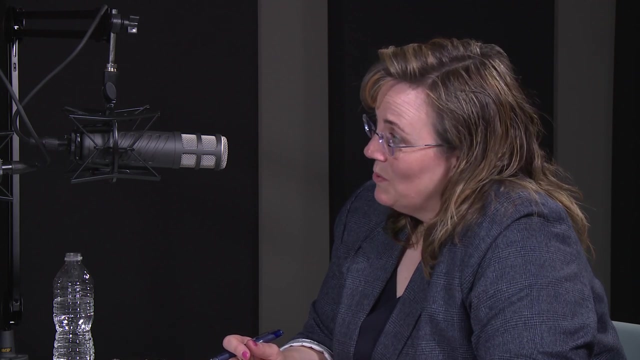 And if there's, if the tools and testing don't find anything, then you've probably done a. you've probably done a pretty good job. So one of the things that Dr Michael McQuaid, the vice president of research here, did in his work with the Defense Innovation Board is cause DOD and others to think about software in different categories. 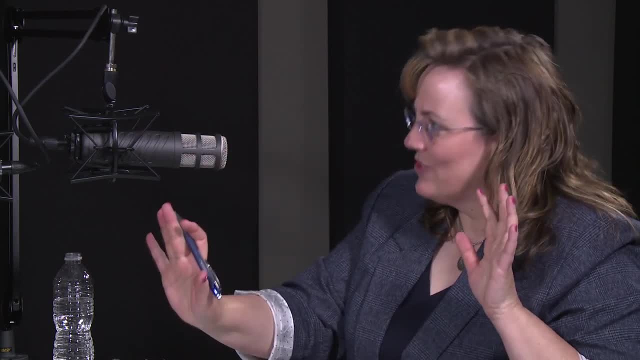 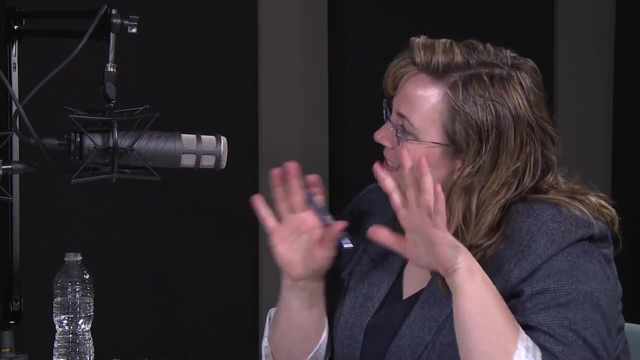 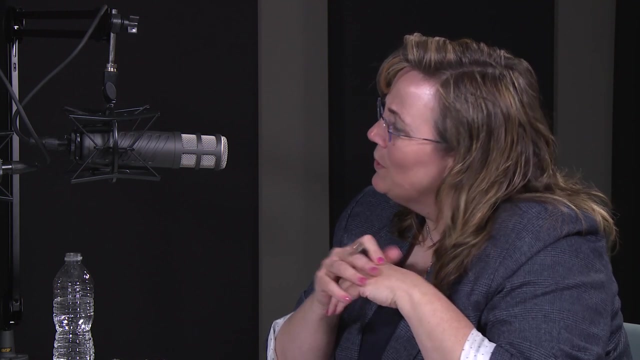 Right. Safety critical software is perhaps different than not safety critical software and apply different methodologies perhaps to those two. Is that a strategy that you know? how do you think through that? Relative to to this, it strikes me that while the requirements are going to be different, in the end the methodology might be somewhat the same. 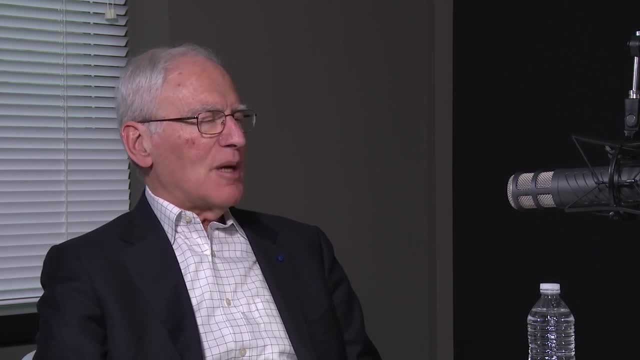 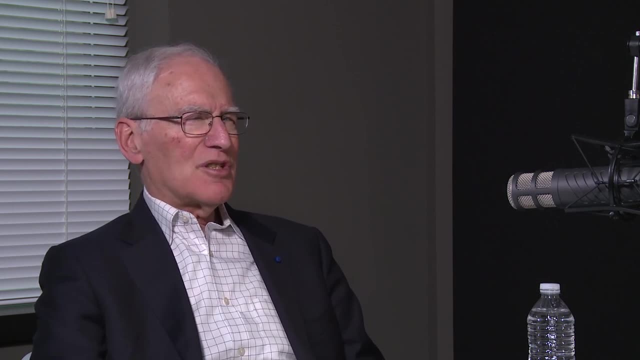 Well, I mean, you know, so you may you know for something. you know something. you know security critical protecting, protecting the nation's most sensitive secrets from the Internet. Maybe you're willing to pay the price of doing, you know the sort of compliance thing. 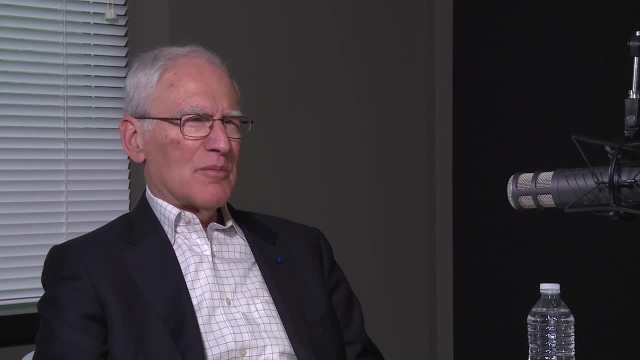 Right And the post testing. But for an awful lot of systems- most systems and most software that runs anywhere- you know where people consider their information important or private or sensitive. I mean you really have to do a base level of secure development because what we've found is that you know I mean vulnerabilities in odd places can result in bad consequences. 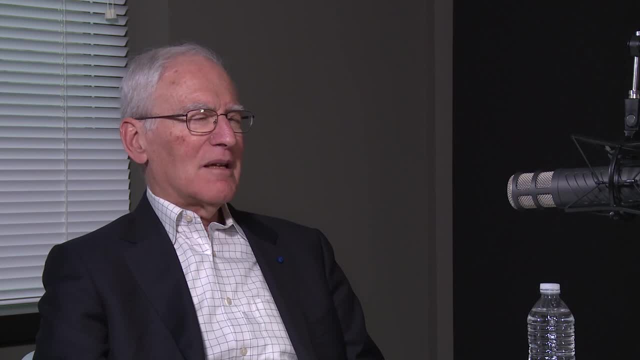 So so I'm, I mean, I think, I think, I think that you know, one of the challenges is we really, we would really like to see, see secure development processes, secure development practices be pervasive or universal or close to that, as we can get them. 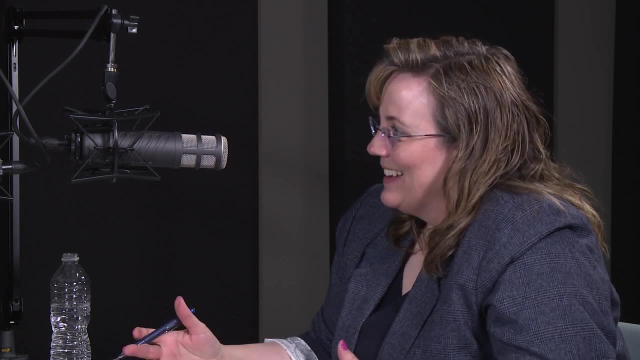 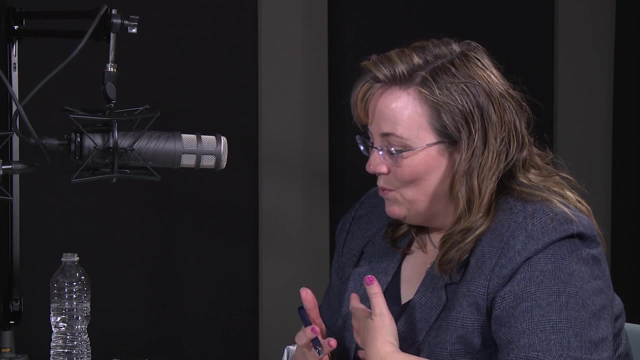 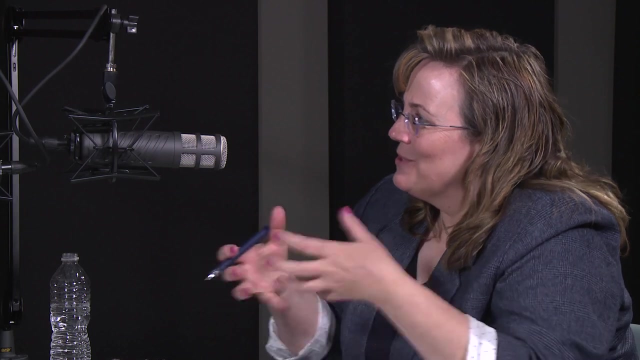 How we write software has changed so much in the last I know from when I learned eons ago, And so how do you think, How do you think about what tooling or what's important for developers today in how software is developed today? Is there some 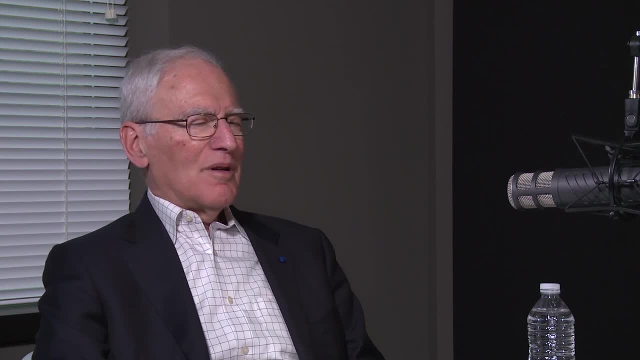 I mean the the main thing. Well, so you know so. so one of the one of the challenges when we created the SDL at Microsoft, I mean we worried initially about C, C++ and C sharp. You know the three sort of common languages internally. you know today, 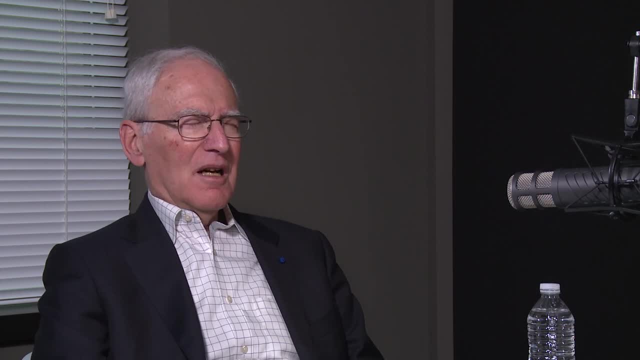 Many organizations that are doing development, you know, are dealing with eight, 10,, a dozen, 20 languages, and you have to do secure development in each of those, And so you know I talk about, talk a lot about scaling. 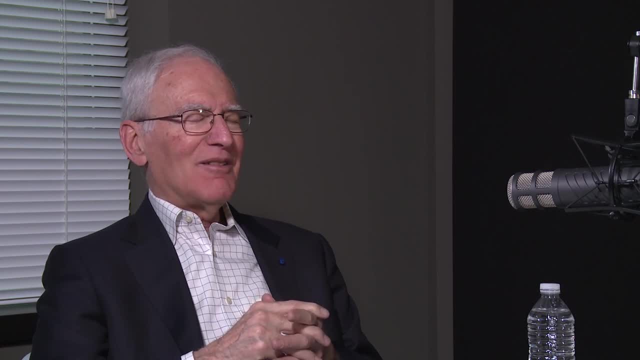 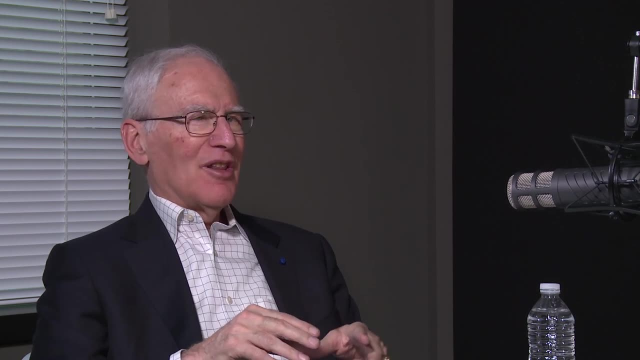 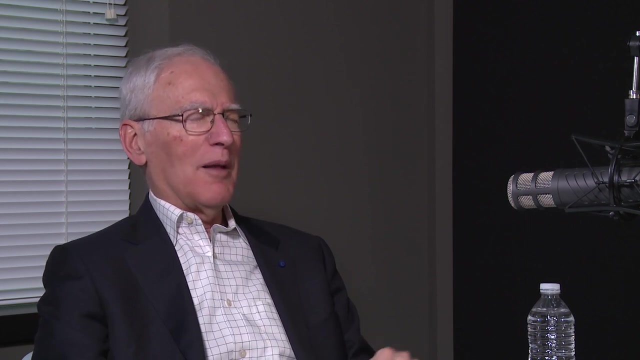 That's. that's a problem. that really kind of poses a scaling problem. The more languages and frameworks you're dealing with, the more different secure development tools, The more tool sets and standards and practices and training you're going to have to have. and if you're a small organization dealing with with 20, 20 or 30 languages or or or or frameworks, you know that that can get, I don't know, overwhelming challenging. it's a problem. 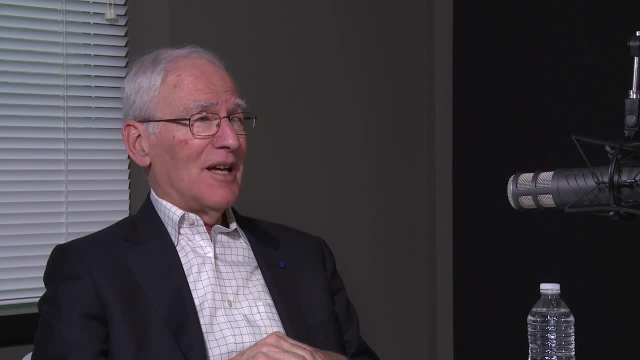 But but you know there's not much of an alternative. at least you know we're starting to see the emergence. I mean you know there's static analysis tools. I mean you know there's static analysis tools. 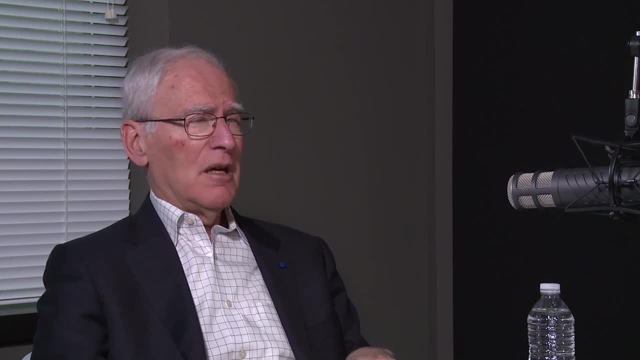 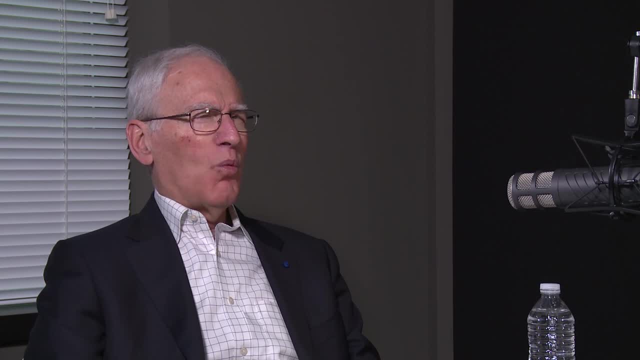 And you know what do you need to do. Thank you. You know what's your standard for deciding whether to accept that or not. you know what to do. You know the SafeCode third-party components document that we released, I guess, a year or two ago, talks a lot about you know best practices for third-party components. 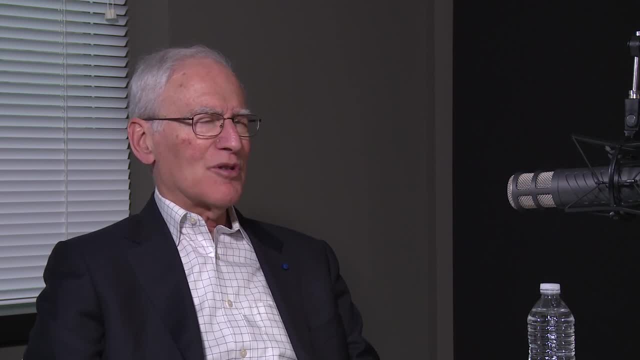 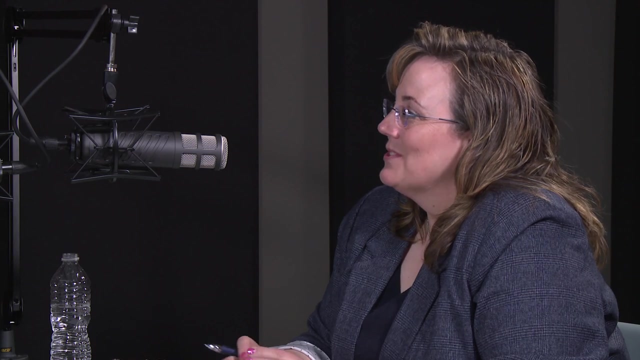 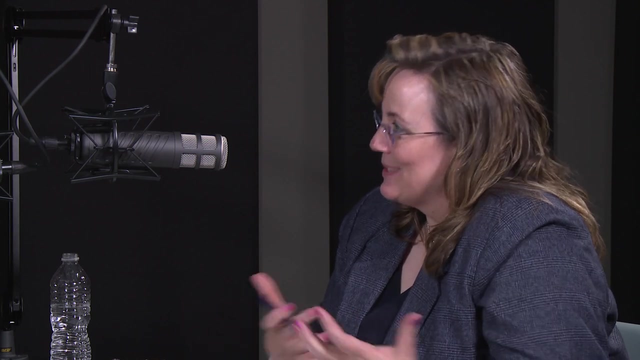 But you know, ideally you'd like your third-party components to be written to as good a security development process as you have yourself. It's not always the case, but that's what you'd like to aim for. Yeah, the supply chain has gotten much more complicated, both in terms of what you're getting, where you're getting it from, how much transparency is or isn't in that supply chain. 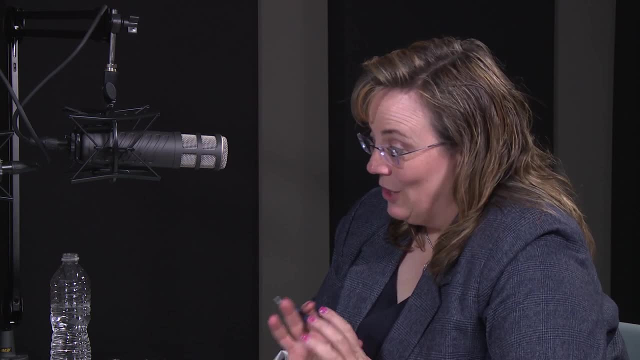 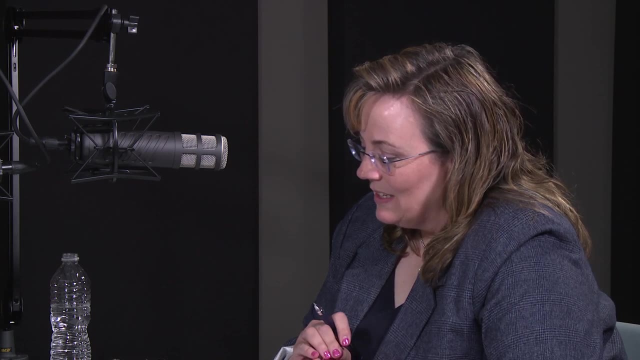 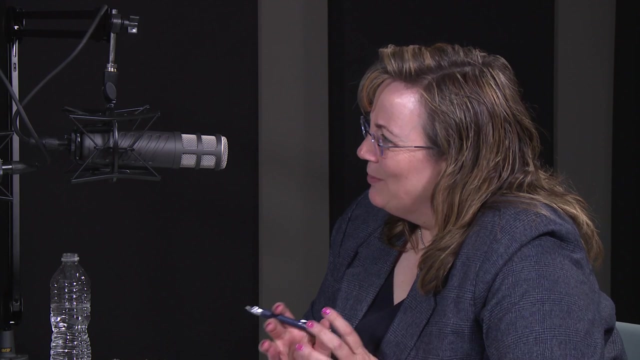 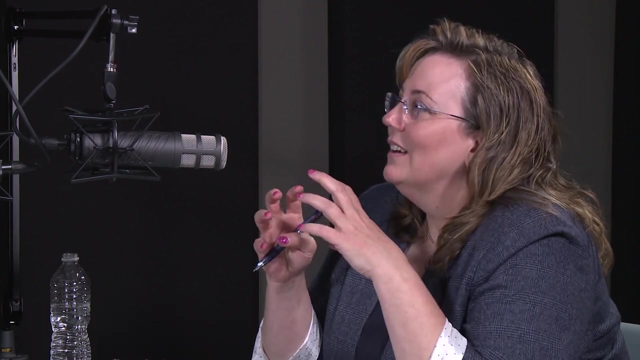 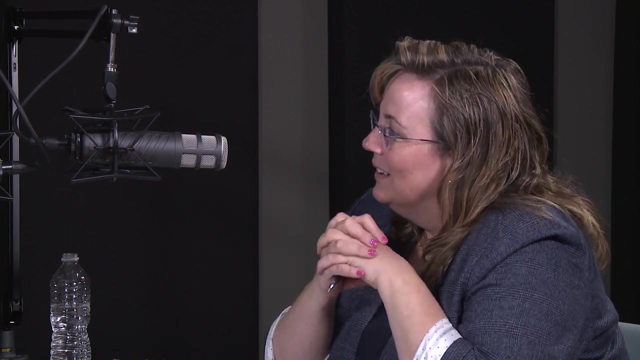 And so I think about that a lot. We think a lot about that. One of the things that I find really interesting is this push for speed. I think speed changes security a little bit in terms of how long something might be at risk, And so how do you think about what we're doing with agile methodologies and DevSecOps and how that aligns with the work you're doing in software? 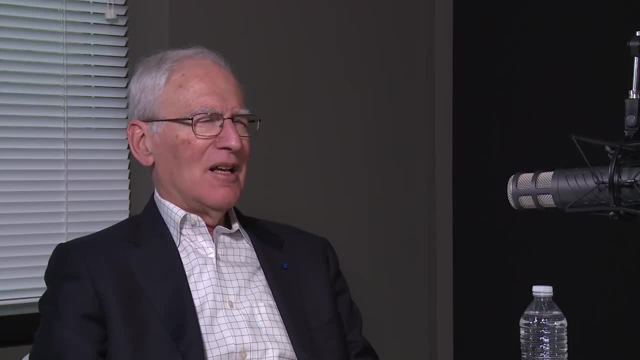 That That came up and I had to face that actually with the MSN group at Microsoft because they were, you know we'd come out with this SDL thing, the secure development lifecycle, And you know they said, well, that's all very well if you're doing a Windows release that's going to ship in three years. 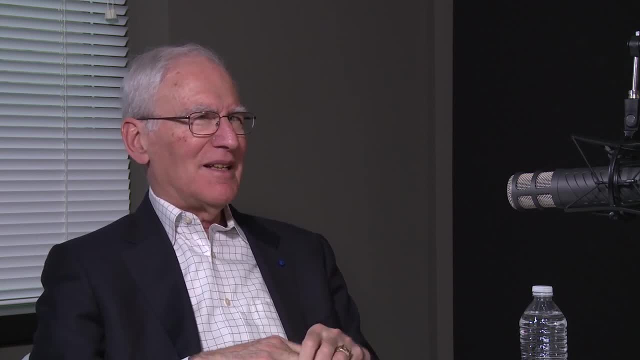 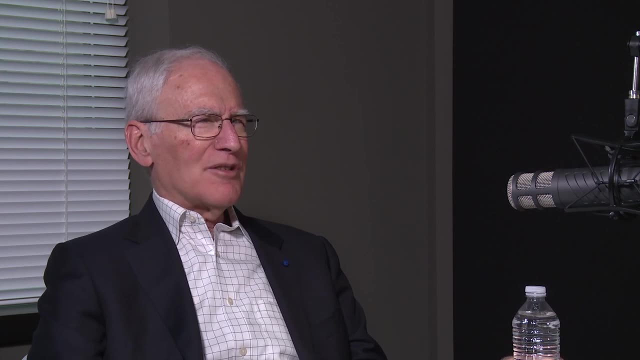 But I'm shipping this afternoon What you know, I mean, it just doesn't work for me. So we actually had a program manager named Brian Sullivan. He knew something about, knew a lot about agile development, knew a lot about the SDL. 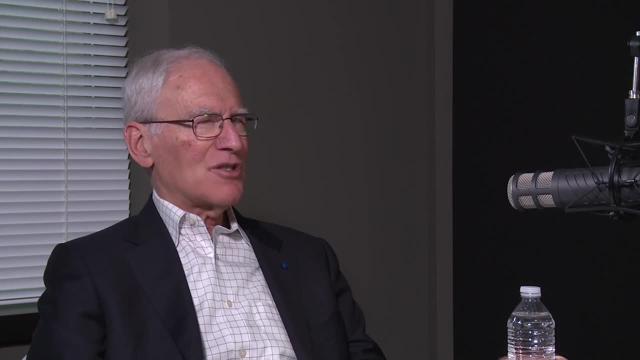 And he sort of thought about it and he enabled us to sort of take the things that we said you had to do and then chop them up, parse them up. So there are some things. if you're, you know well, you're shipping this afternoon, that's fine. 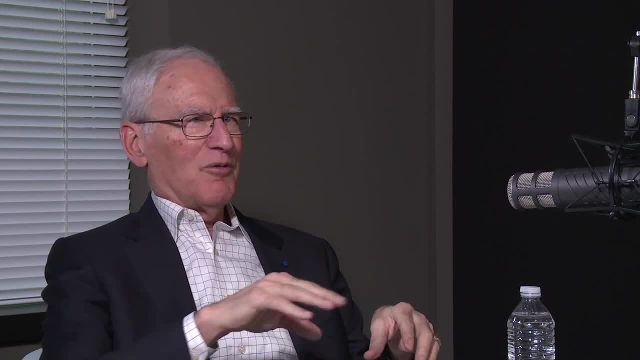 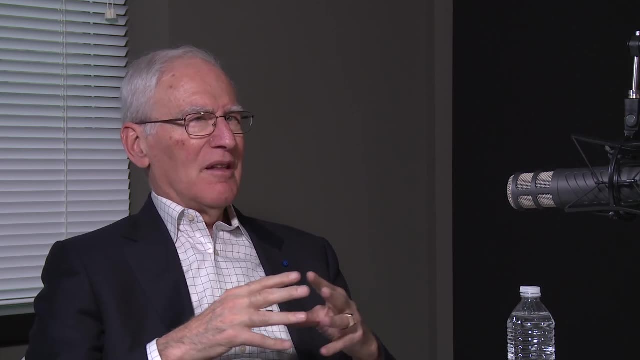 But you still, your code still has to run through your compiler tool chain before it gets deployed. So there are some security, There are some measures, some tools that can just be integrated into that tool chain and their SDL requirements. So you just meet those as you go, every time you ship. There are some. you know, if you're doing the broad architecture, the design of a system, maybe that's something you're doing at the beginning of a project And then it's only a major rev where you reconsider that. So if your threat model, you do that once you've probably got a threat model that's good for a while. 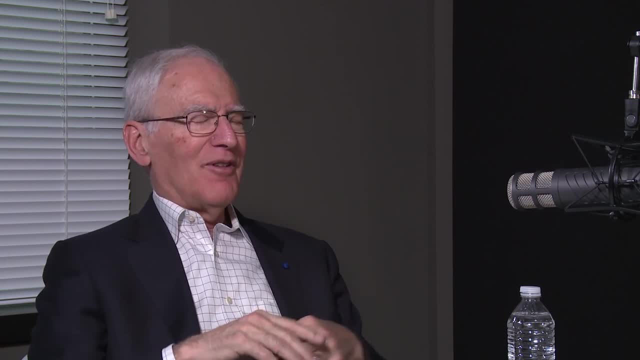 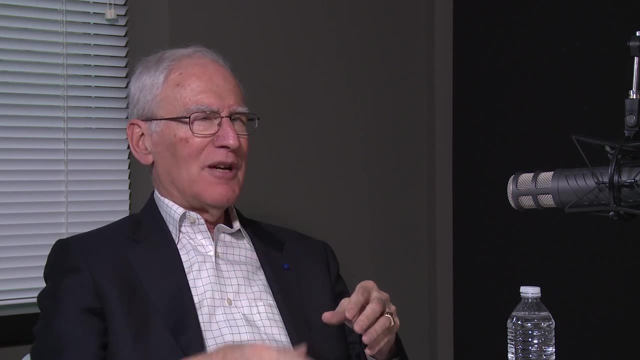 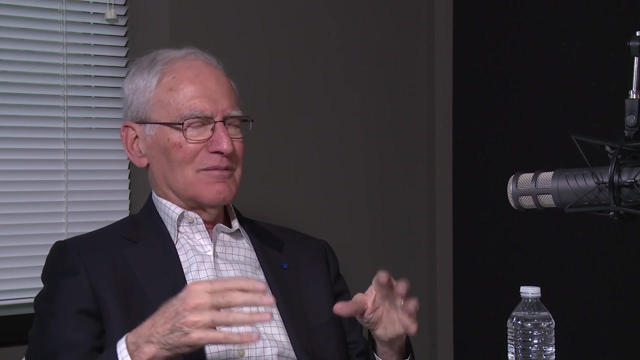 And it sort of tells you what to do as you go. And then finally, there's some kinds of testing that you have to run that take a while to do, And maybe you do those periodically rather than doing them. you know every after. you know doing, you know three days of testing every afternoon. 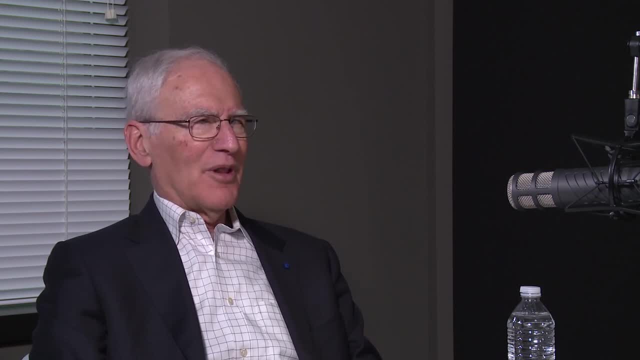 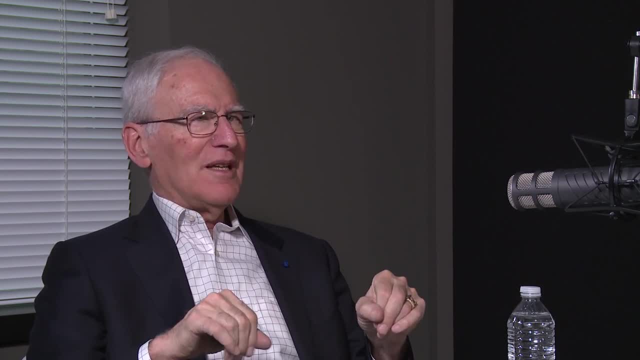 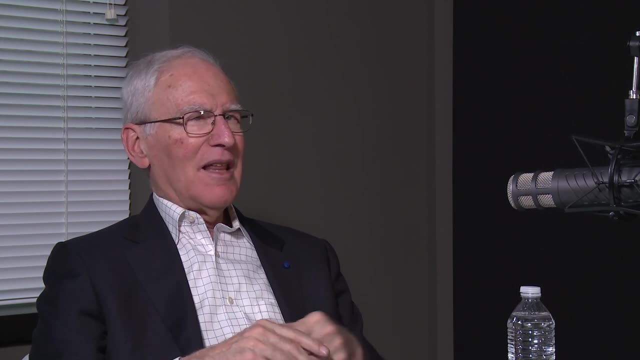 Right, Right, Right, Right, Right And overall that process was how we tackled agile security for the agile development cycles And that worked out pretty well for us, And I think probably that same model applies even. you know, DevOps, DevSocOps, what have you, if you just think about parsing things out that way? 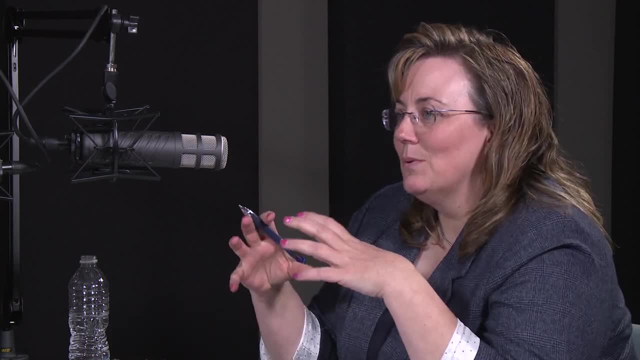 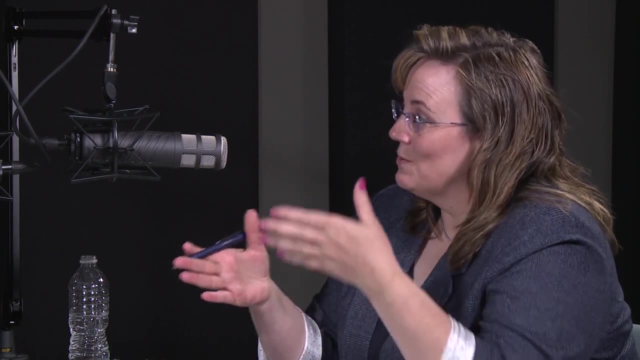 Yeah, The interesting thing to me is the potentiality. with all the tooling today, Okay, I mean you can get data that can then be used and you can push your risk management earlier in the process. You can push your security arguments earlier in the process. 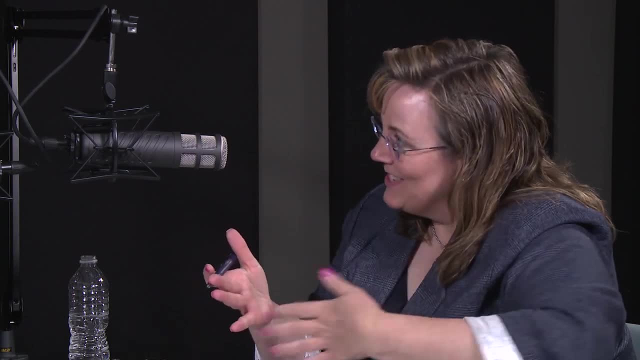 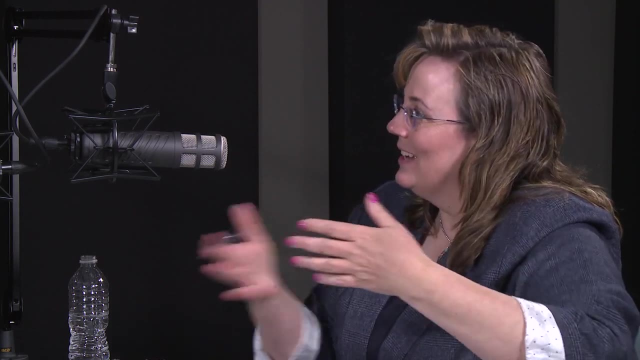 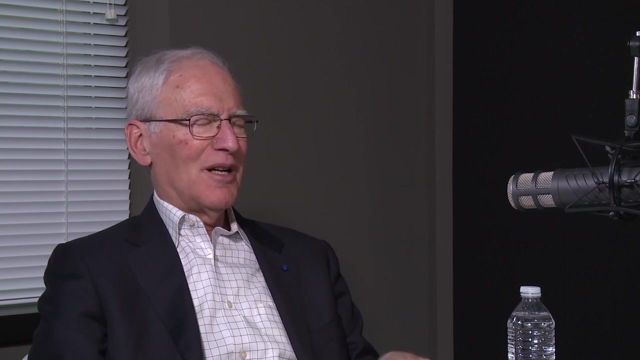 You can push your validations earlier in the process And, as you can speed up the release of hopefully ever-improving quality, unassured software, you can change a bit of the dynamic If you can get the tools and if you can integrate them into your development. 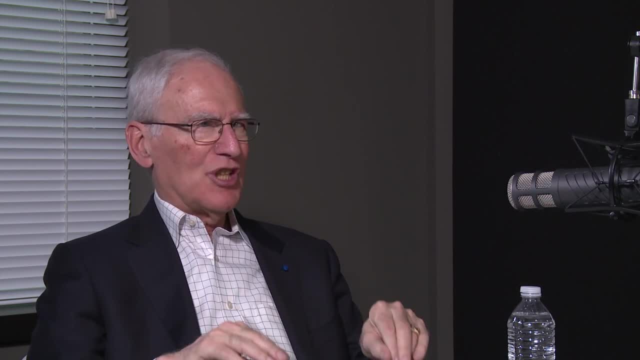 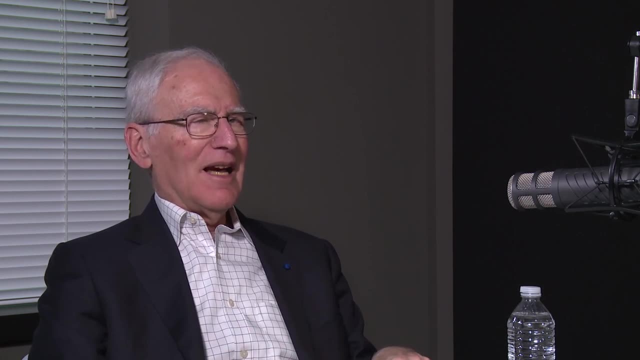 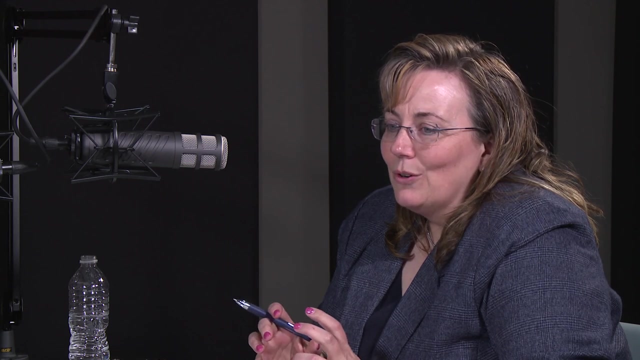 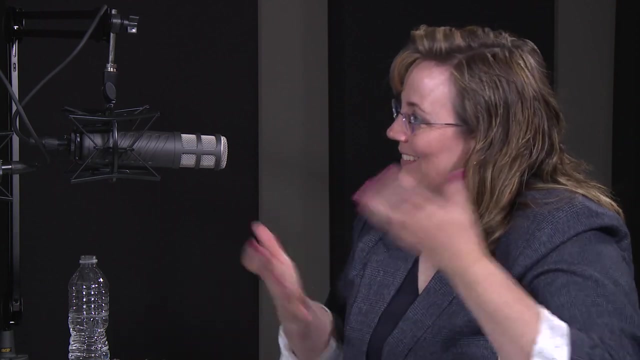 If you can develop- you know, developer desktop or development chain- then that's. you know, that's a great way to get the assurance up and the residual vulnerabilities down. And it'd be interesting if we could get to a point where your third-party software has some data from its tooling about it that you can then incorporate right. 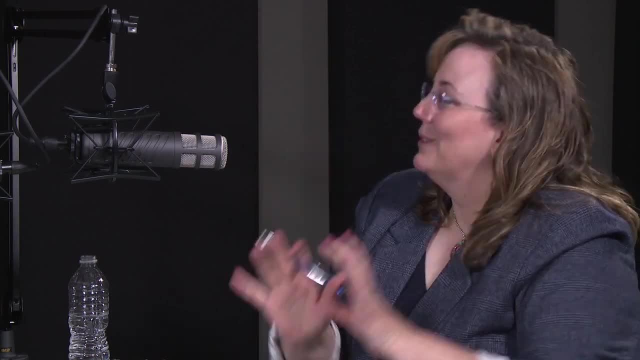 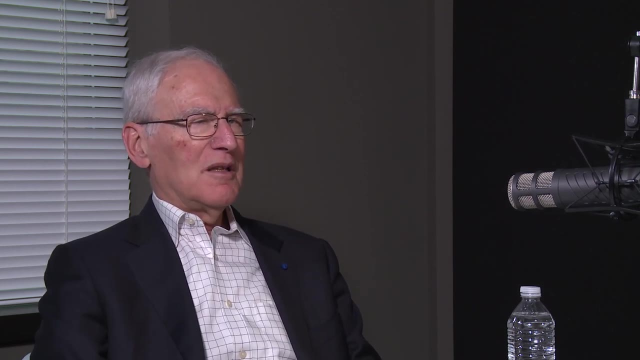 There's a little bit of a vision out there that we're all working towards. That would be it. That would be it. That would be a great vision if we could realize it. I'm sure a lot of organizations would be very happy to know that some you know coding best practices, that some static analysis had been run on the third-party components they were consuming. 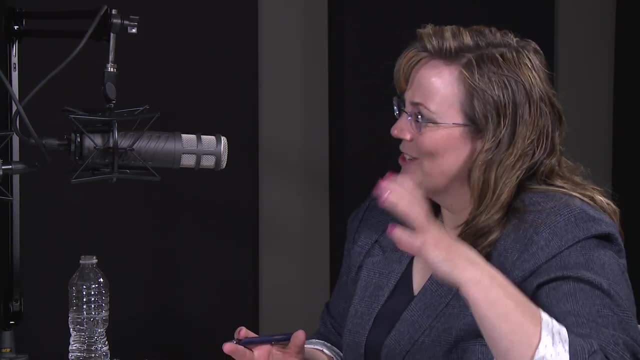 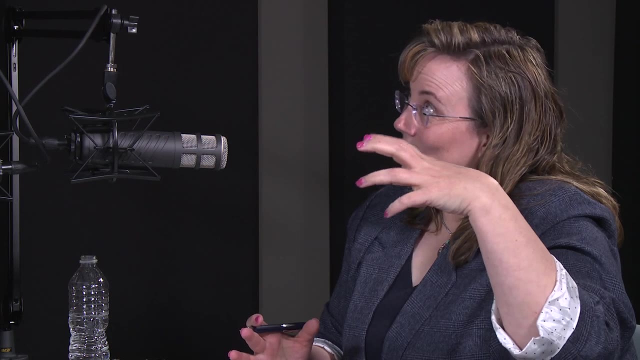 Yeah, And I think that's some of the software bill of materials activities: trying to see, at least knowing what's in there, And then the next step about: could you put some details about the what, what, the quality standards of the thing and other? 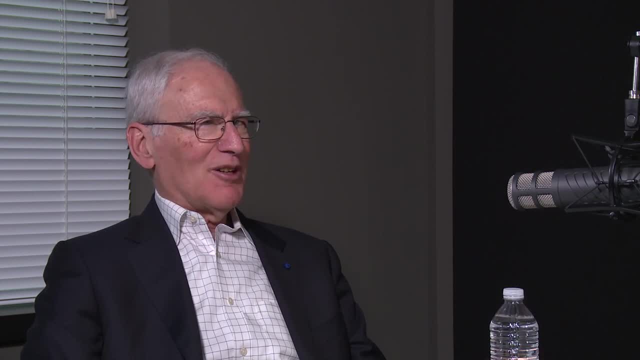 Yeah, I'm, I'm, I've been, I've been a little bit of a skeptic on the software bill of materials. I think it is super monumentally important for developers to understand their bill of materials and what they're using. When people say, you know, end users need to understand the, the bill of materials, you know, I, you know, I sort of, I mean, I sort of ask why and what are they going to do do with it. 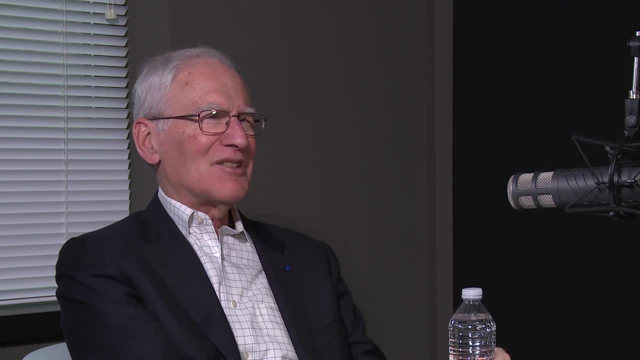 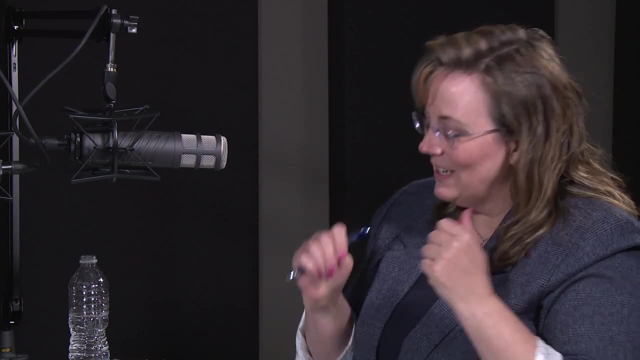 I mean, that's, that's sort of a harder, that's sort of a harder case. For me, the utility is in the architecture and the design, design and the implementation at the development stage. I, I, I hear your, I hear your comment. 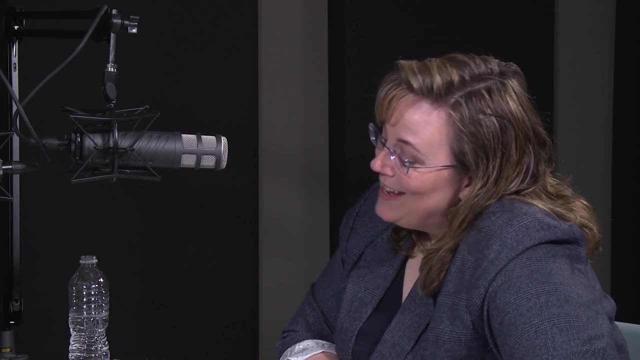 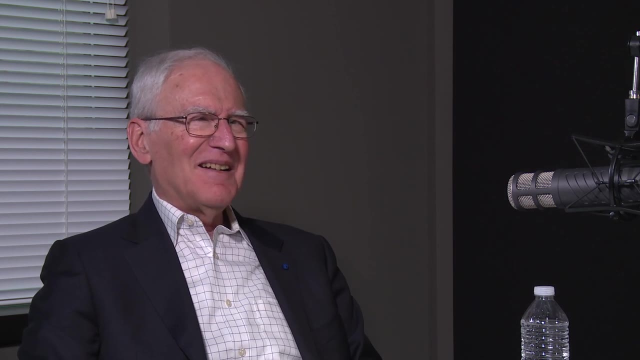 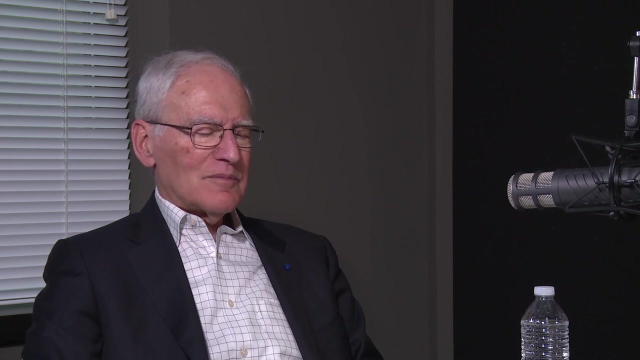 So one last question: What do you know now that you would have liked to have understood much earlier? Oh gee, So so I guess I guess what I need, what I what I know now That I would have liked to have understood much earlier- is that you know, getting getting to secure products, getting to software security, is really a matter of of continuous improvement and and and root cause analysis, rather than trying to build the perfect model and then work for decades to to implement it. 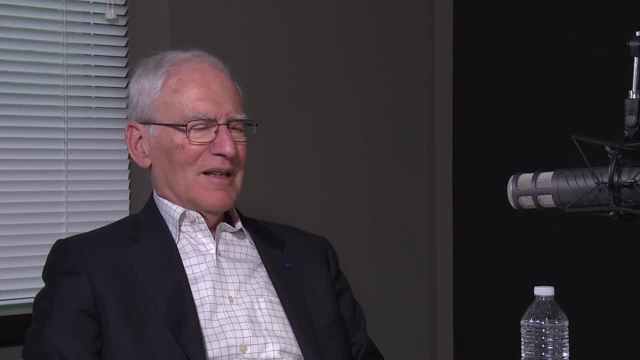 There, there. there are cases where people- Well, there are cases where I mean, I've tried the perfect model, and, and, and it didn't come out so well, But you know, and, and there are people who still believe that that's what we ought to do, and in another 10 years it'll all be nirvana. 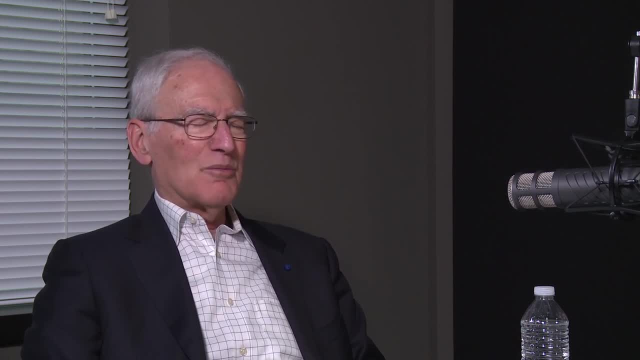 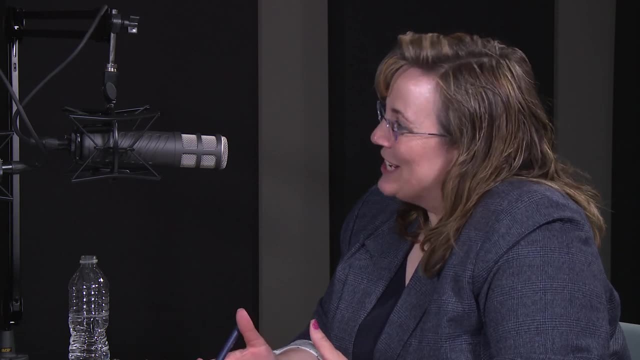 But but I think I think if I can do continuous improvement for 10 years, things things will be a lot better. Yeah, it's a thematically right, it's a culture change question. I've heard you say: 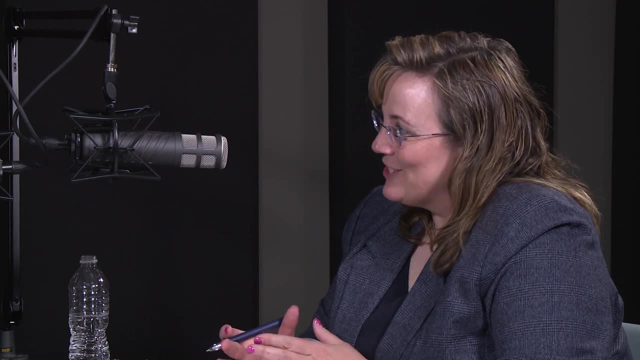 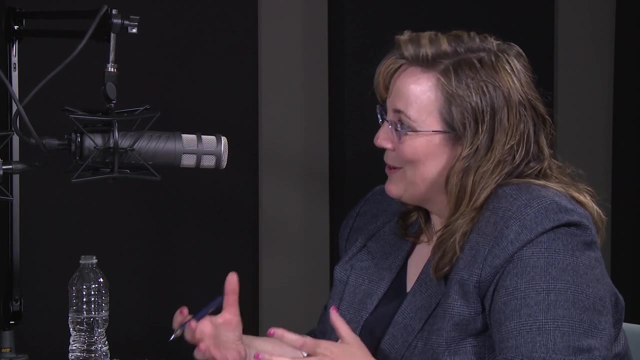 Yep, yep, I've heard you say: hit the point of best impact For intervention. the developers and the and the software, think about good design patterns and threat modeling and other approaches to do it and constantly improve as you're going along. Constantly improve Every, every vulnerability report. you take a vulnerability report, you do a root cause analysis, you're out. why did that happen? What can I do, not just to fix that vulnerability Right, But to fix it and all its friends and relations? 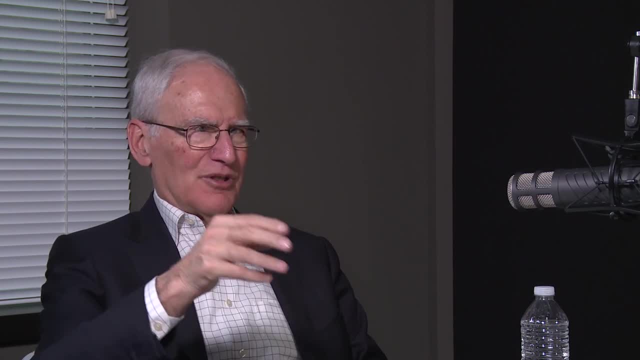 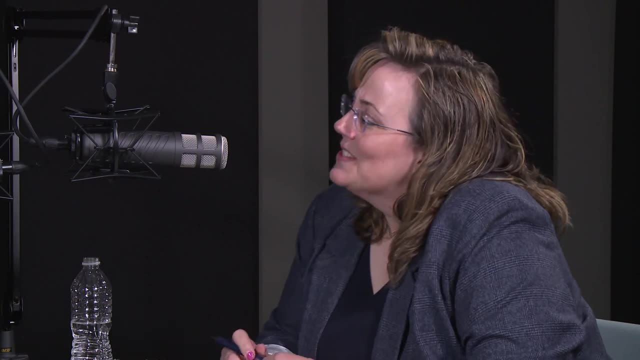 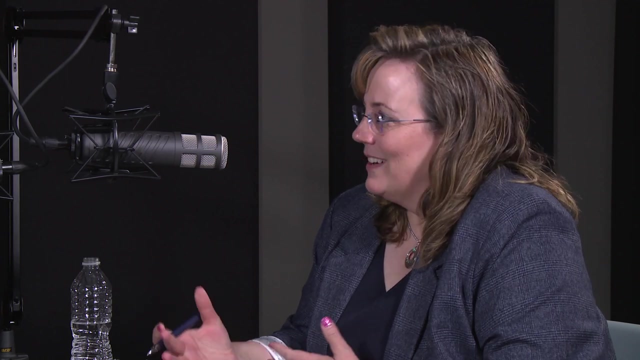 And you just keep cycling that and over time you just turn the knob up and up and up Right and frustrate that, that situation. So, ultimately, culture change is a big issue for security and it strikes me that the work that you took on at Microsoft- and you know, you and I met, I think, the first time when you had just come to Microsoft and I was still in the DOD- 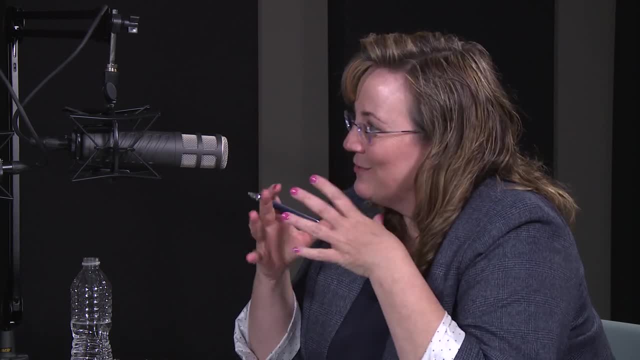 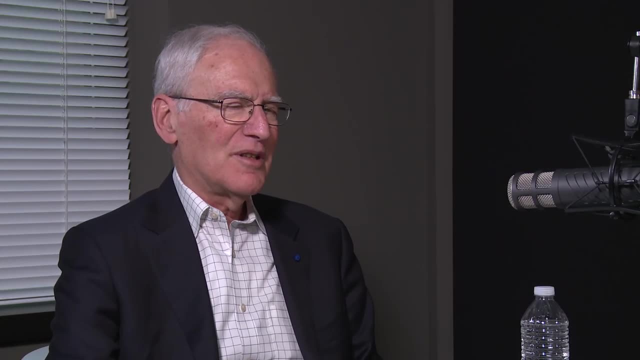 How can we change this corporate culture to focus on product security? How, how did you build that? How did you go about that? So for us at at Microsoft, the big turning point were- I think were were- two things. 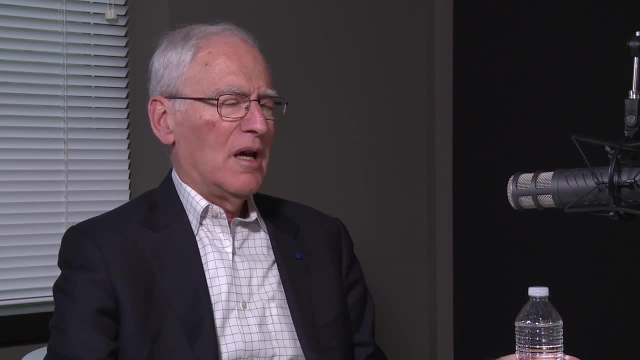 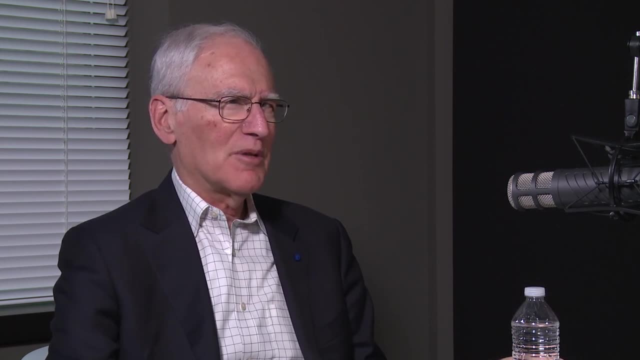 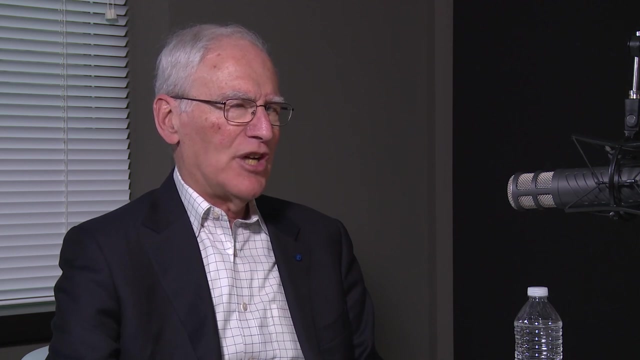 One of them was the- you know all the problems we had in 2001 that that we talked about- And the other was the, the trustworthy computing commitment, the trustworthy computing email that Bill Gates sent, And that was a combined project of Bill and Chris. 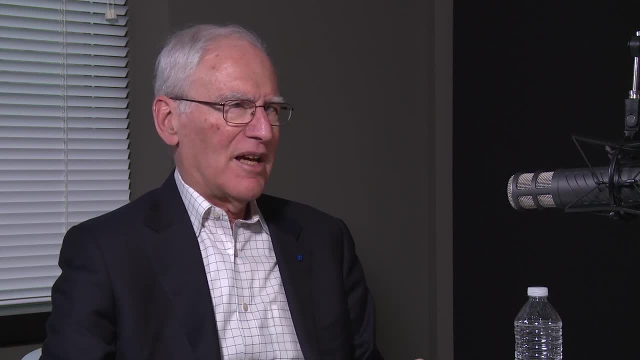 Craig Mundy, who was one of our CTOs, and the late Howard Schmidt, late, great Howard Schmidt, who was my predecessor at SafeCode and at the time had been the chief security officer at Microsoft. The three of them- Howard, Howard and Craig- really pushed, you know, encouraging Bill to, to create the, the TWC commitment and make that part of the company. 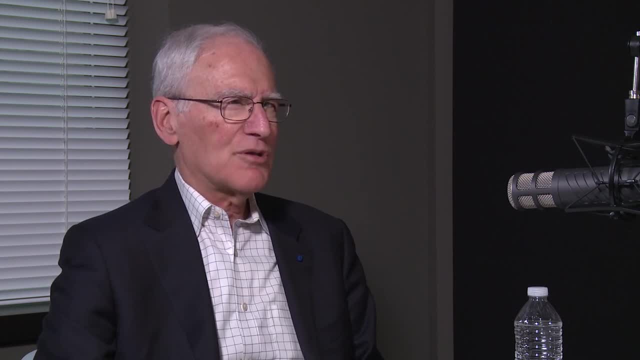 And that sent the message across Microsoft And to the working level developers. this was something we were serious about. Other thing, sort of an interesting story about that: We as part of the you know starting this Windows security push and and doing the focus on Windows Server 2003,. we trained everybody. 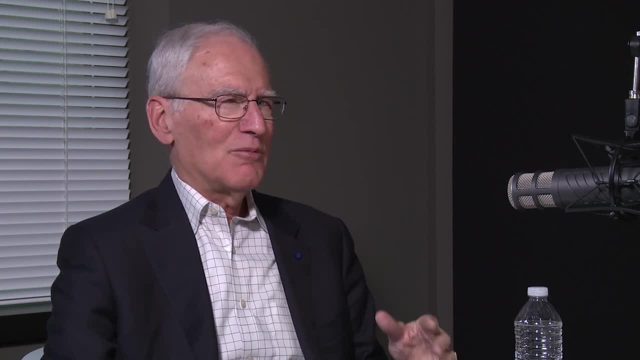 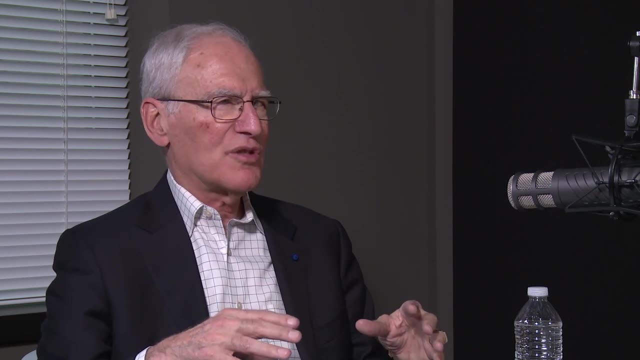 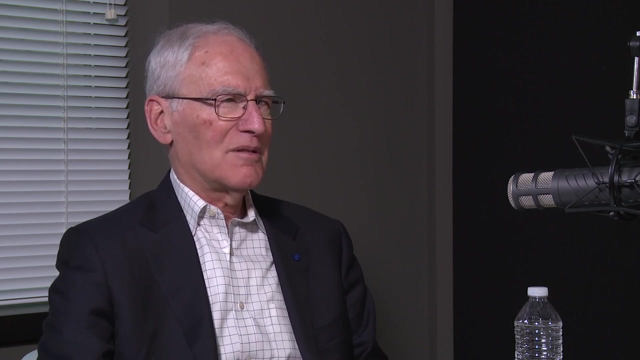 We had a room that held a thousand people. We trained them in blocks of about eight or nine hundred, ten times in ten sessions over the course of a week. for our session And for each of those sessions we had a corporate vice president, one of the the inter intermediate level managers in the Windows division, come in and introduce the training. 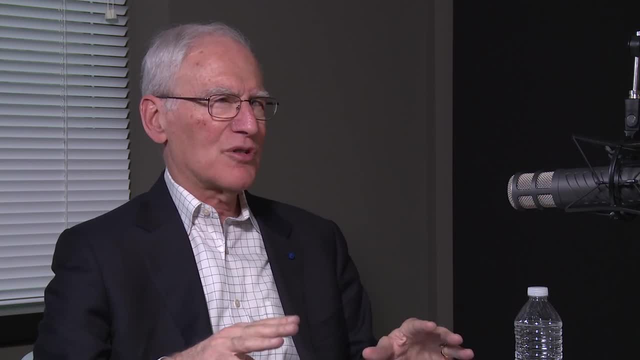 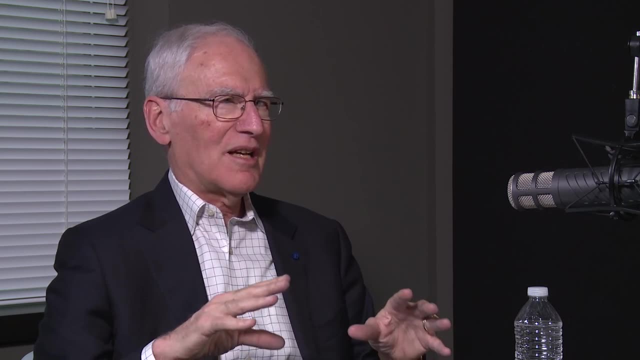 Okay, And if you've done corporate training, you know how that works. The the corporate VP comes in, introduces the topic, tells you why it's important and then leaves- Okay, In the case of the Windows security push training corporate VP came in, introduced the topic. 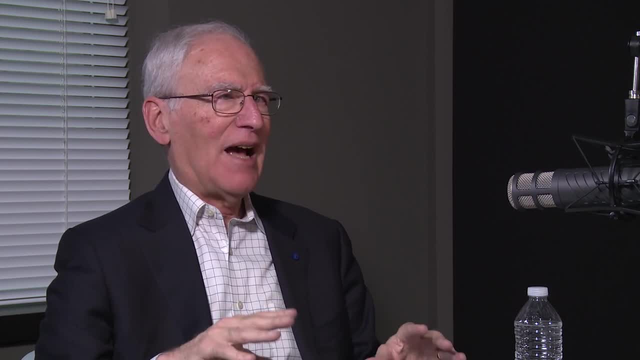 Told everybody, Told you why it was important, And then sat down to take the training- Oh wow, And that you know that's a. that's a message you don't see in companies very often. It kind of tells you what's important and what's not. And I think that worked for us pretty well too. Yeah, so allies from lots of places really pushing forward and corporate leadership attention, These people's VPs, these people's managers. you know this is important enough for me to spend four hours of my time learning it.